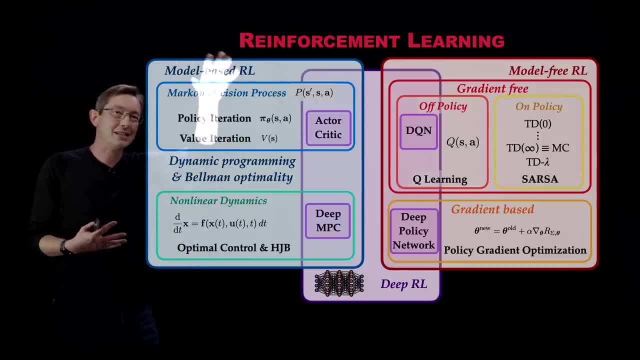 going to be specifically talking about model-based reinforcement learning. This has a really rich history in optimization theory, dynamic programming, non-linear dynamics. A lot of this came about from Richard Bellman's Bellman optimality condition and dynamic programming. So Bellman. 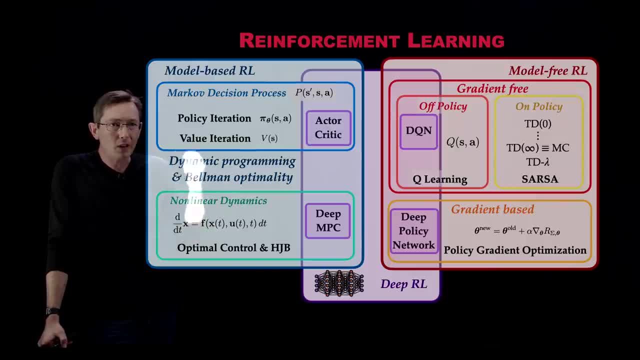 made a huge, huge impact to the field coming up with these kind of optimality problems, showing when you can solve sub-problems and still get a globally optimal solution, and those are still being used today in these policy iteration and value iteration algorithms. 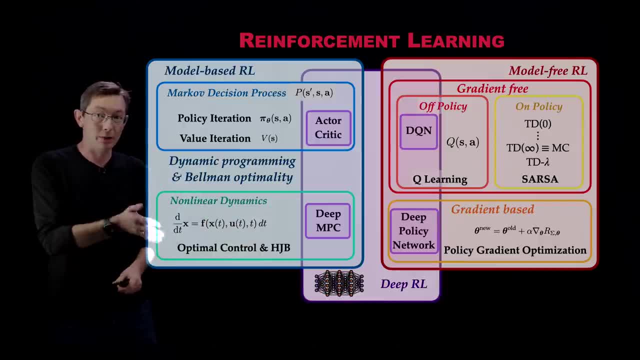 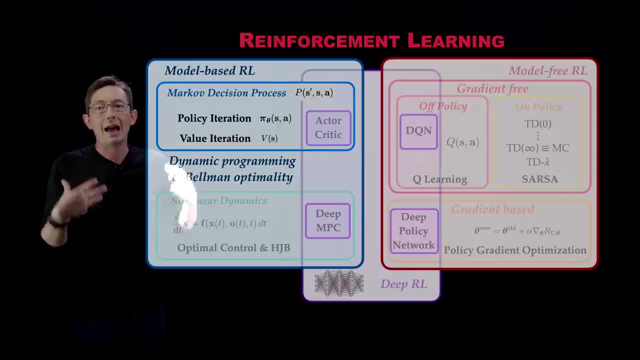 and in optimal non-linear control using the Hamilton-Jacobi-Bellman equation. So, specifically today we're going to zoom in on this block here, and so we'll be talking about how do you kind of iteratively optimize a policy or a value function by solving sub-problems. 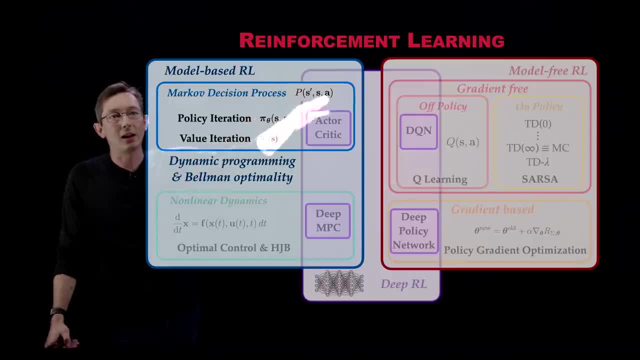 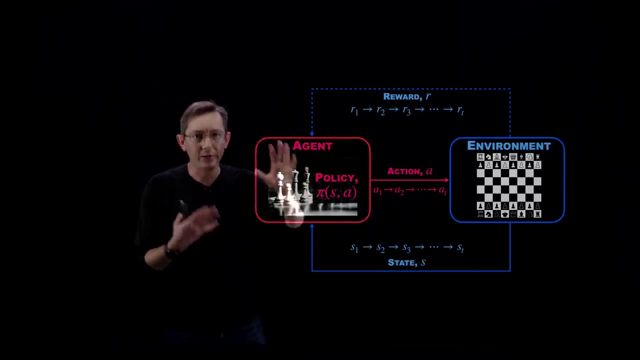 with dynamic programming, And so this is in the context of a Markov decision process. We assume that our agent is interacting with is a Markov decision process, so some probabilistic state transition process. Okay, and I'm going to jump in To give you the details of dynamic. 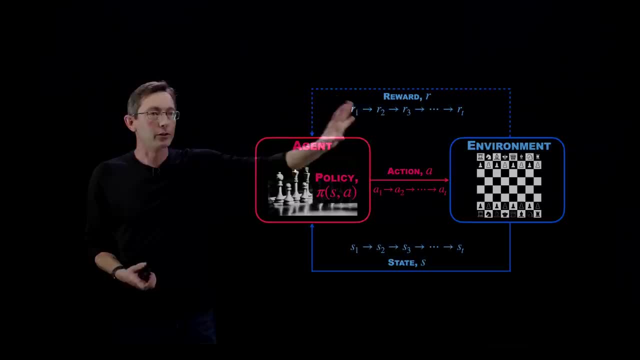 programming and policy iteration and value iteration. I first want to just recap the really, really basic stuff for reinforcement learning in case you're just tuning in. So our agent is interacting with an environment. It senses its state through a series of measurements, S at time one. 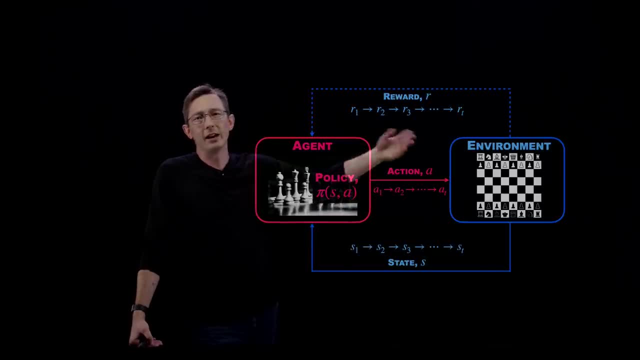 Time two, time three. this is an iterative measurement process. We're assuming a discrete system like playing a game of chess, where it's turn-based And at each time I get to decide on an action, to take A to try to hopefully maximize my future reward for this game. 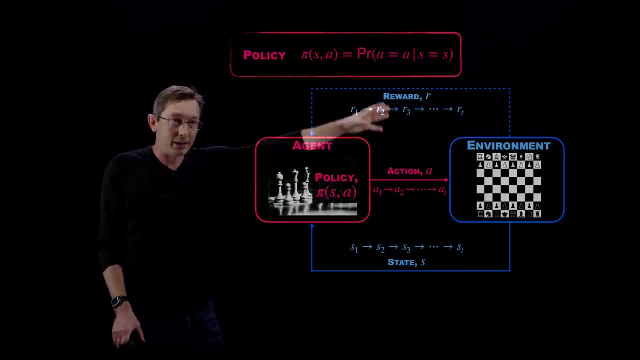 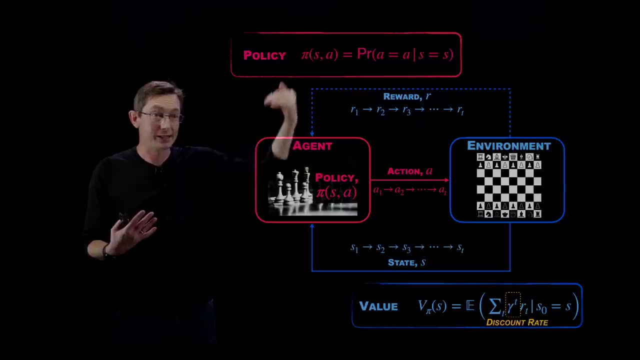 And we are trying to design an optimal policy pi again that gives us the maximum future rewards. We have this value, function V, that, given our policy pi, it tells us how advantageous is it. What is the expected future rewards of being in this state now and enacting 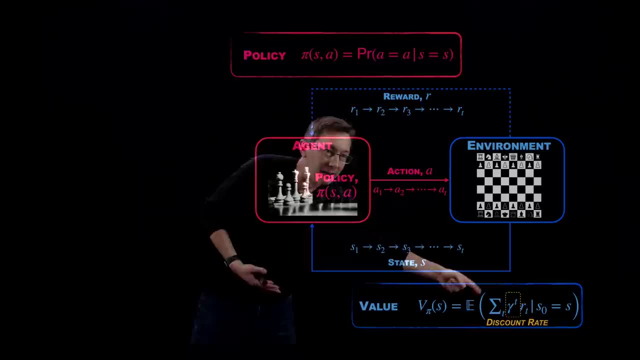 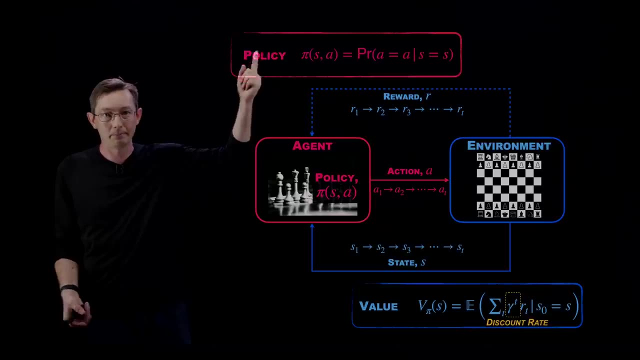 this policy pi And it's a probabilistic process, so we're taking the expected value of our future rewards given some policy pi And I don't know the best policy or the true value function for that best policy, out of the gate. That's what I'm trying to learn. I'm trying to learn the optimal. 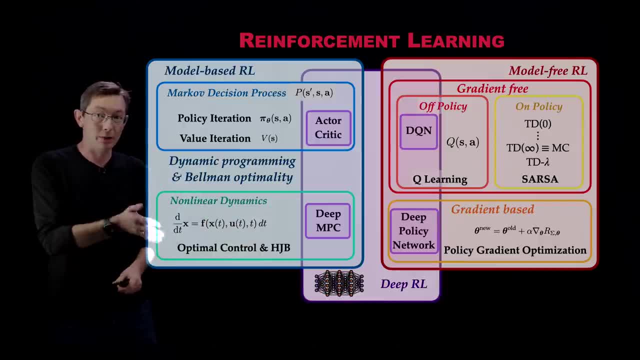 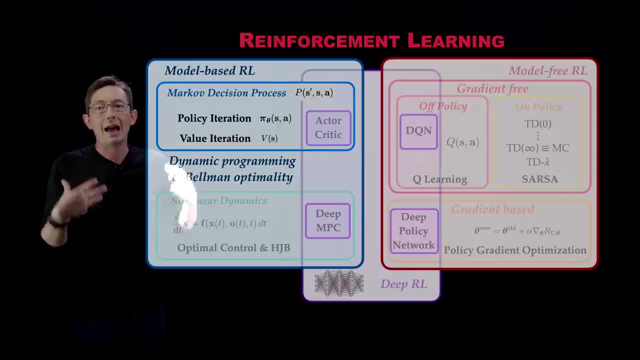 and in optimal non-linear control using the Hamilton-Jacobi-Bellman equation. So, specifically today we're going to zoom in on this block here, and so we'll be talking about how do you kind of iteratively optimize a policy or a value function by solving sub-problems. 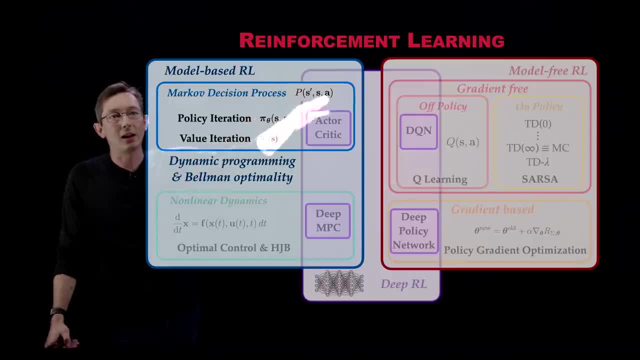 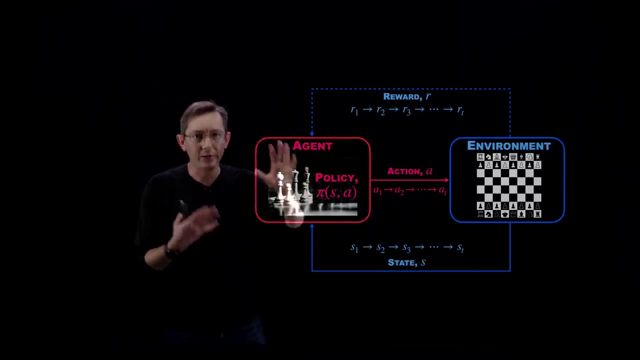 with dynamic programming, And so this is in the context of a Markov decision process. We assume that our agent is interacting with is a Markov decision process, so some probabilistic state transition process. Okay, and I'm going to jump in To give you the details of dynamic. 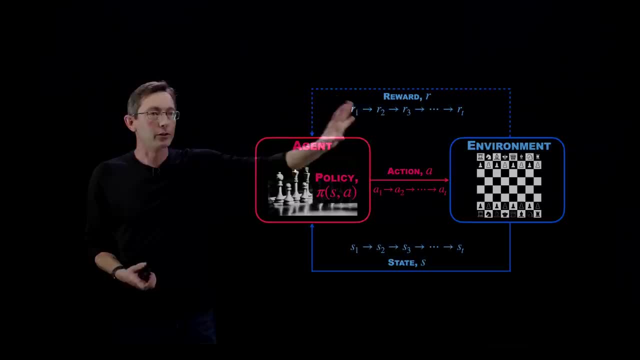 programming and policy iteration and value iteration. I first want to just recap the really, really basic stuff for reinforcement learning in case you're just tuning in. So our agent is interacting with an environment. It senses its state through a series of measurements, S at time one. 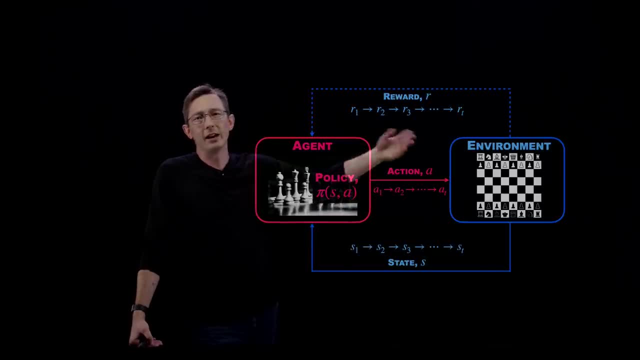 S at time two, time three. This is an iterative measurement process. We're assuming a discrete system like playing a game of chess, where it's turn-based And at each time I get to decide on an action, to take A to try to hopefully maximize my future reward for this game. 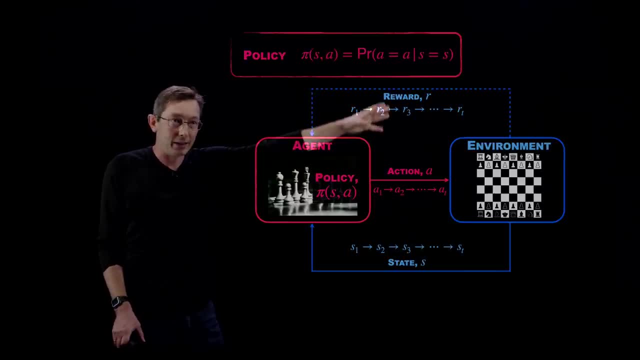 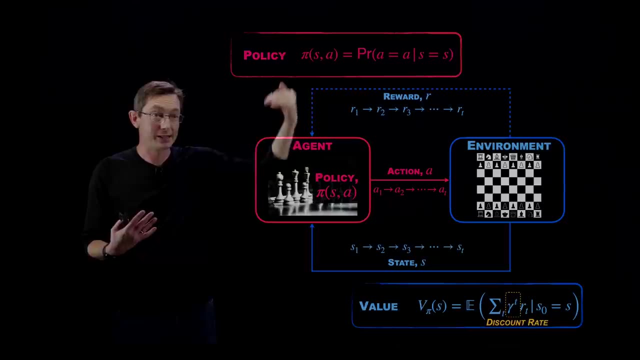 And we are trying to design an optimal policy pi again that gives us the maximum future rewards. We have this value, function V, that, given our policy pi, it tells us how advantageous is it. what is the expected future rewards of being in this state now and 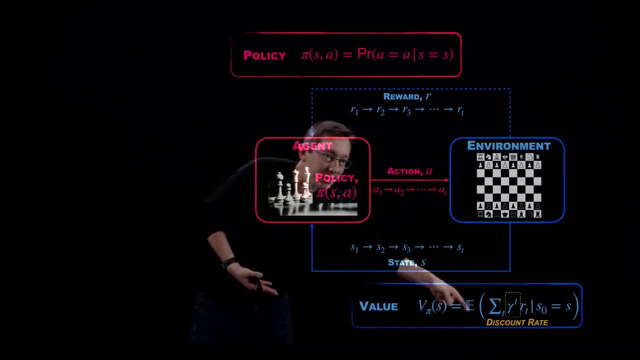 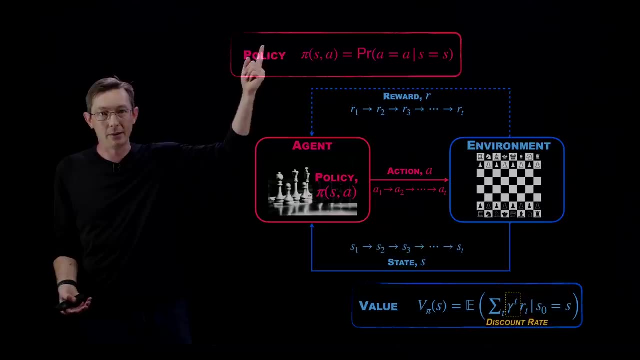 enacting this policy pi And it's a probabilistic process, So we're taking the expected value of our future rewards, given some policy pi And I don't know the best policy or the true value function for that best policy- out of the gate. 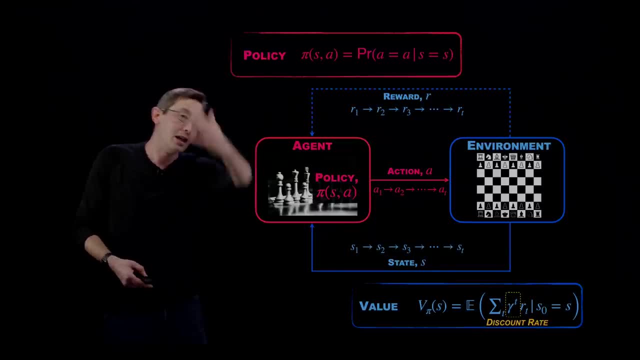 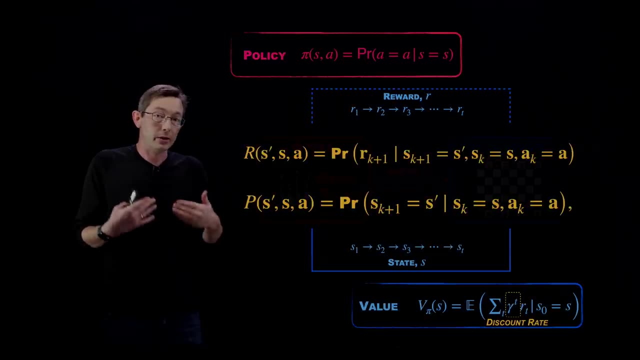 That's what I'm trying to learn. I'm trying to learn the optimal policy and ideally also an optimal value. allows that function for what is the best state to be in What we do? assume that we know at the outset. 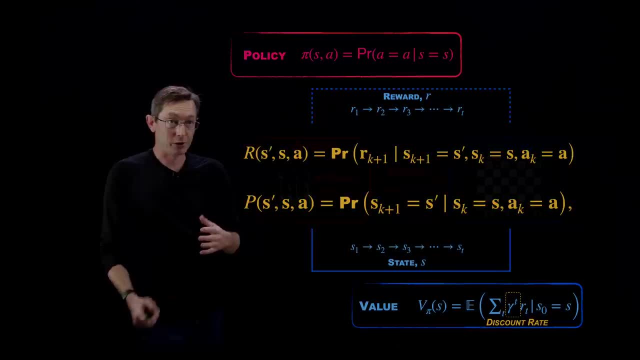 at least for this model-based reinforcement learning. for kind of the simplistic version is: we assume that we have a model for how the environment works, how the system works, So we assume that the environment evolves according to a Markov decision process. So that would be this probability here. So the probability that the state of my system policy and ideally also an optimal value function. So, as I said, I'm trying to learn the optimal policy, and I'm trying to learn the optimal policy and ideally also an optimal value function. But when we're getting into that, what do you want to do? You can't just say: hey, that's enough. You can't do just that. 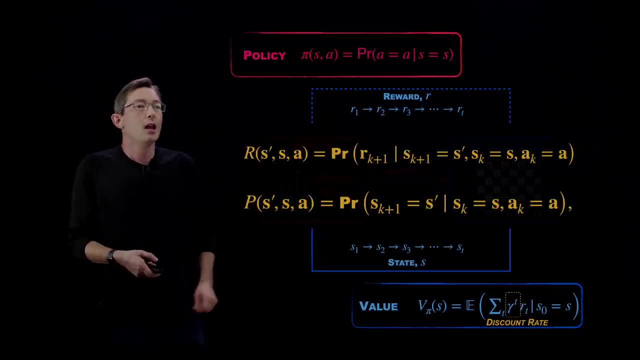 function for what is the best state to be in What we do? assume that we know at the outset at least for this model-based reinforcement learning, for kind of the simplistic version is: we assume that we have a model for how the environment works, how the system works, So we assume that the environment evolves according. 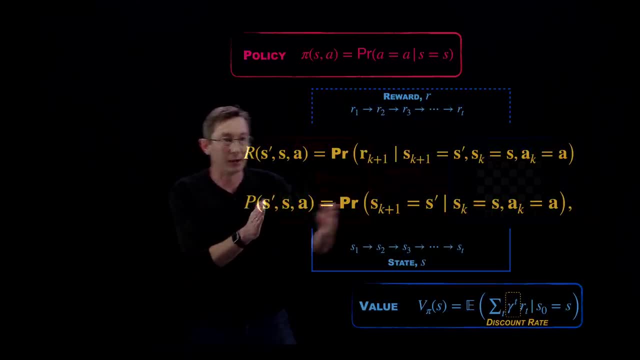 to a Markov decision process. so that would be this probability here. So the probability that the state of my system at the next time step will be S prime is some probability based on or conditioned on my state currently being S and my current action being A. So, given a current state S and a current action A, 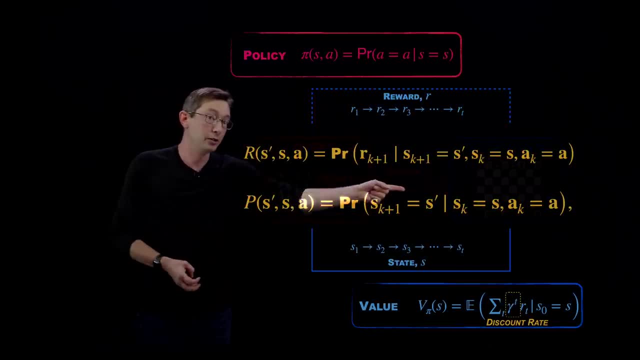 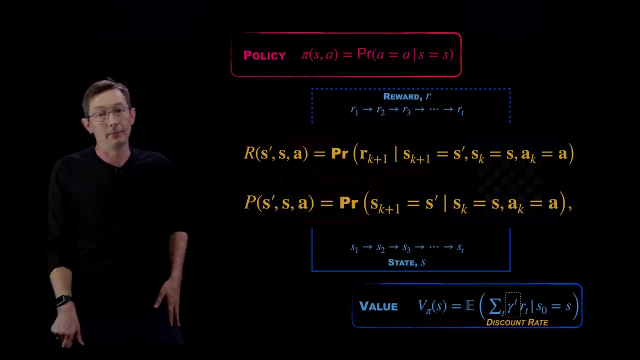 there is some probability that my system will transition to a new state S prime and that's encapsulated in this probability model P. This is called a Markov decision process and it generalizes a normal Markov process to have this action or control input A. 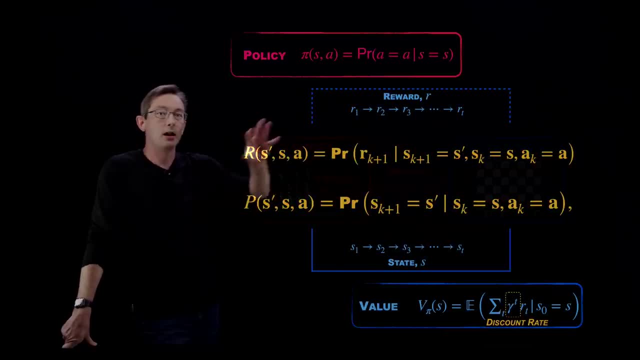 We also assume that we have some model of what the reward structure looks like. So what is the probability of a reward given some current state S or sorry, given a current state S and a current action A, and assuming that I move to a future state S prime in the next state, what is my expected reward? 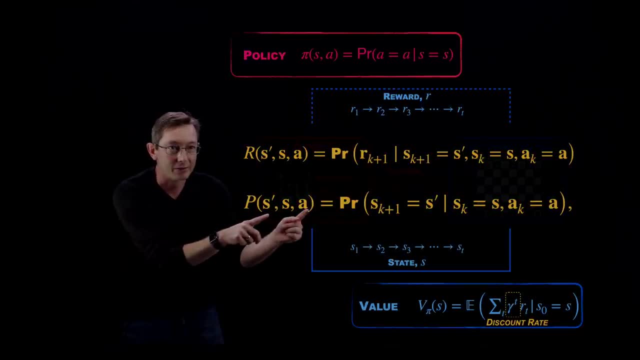 given all of that happening. So, given kind of this information, what is my expected reward at the next time step? And again, this is kind of an assumption- that you know the rules of the game you're playing. So if I'm playing chess, for example, you know the reward only. 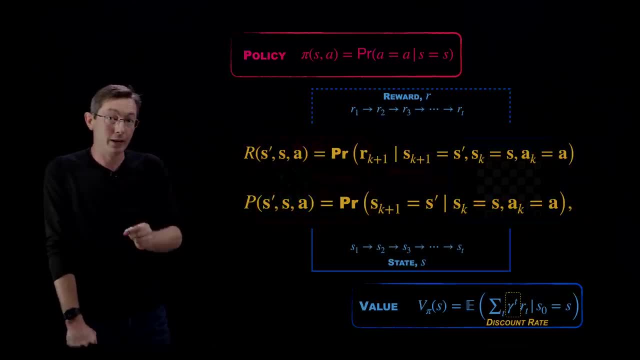 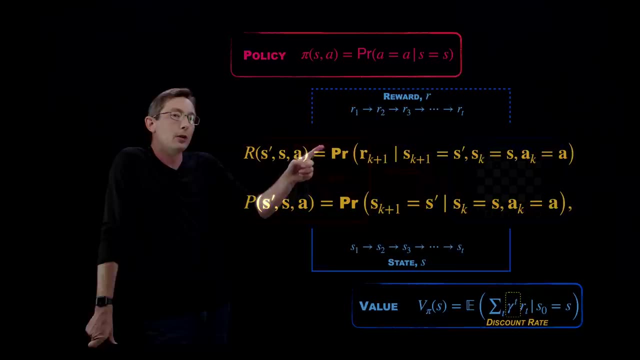 comes at the very end of the game. but I know what the rules to win are. I know how to checkmate someone or how to not checkmate someone. You have to know that going in to play, And so this would basically say I know what my reward is. 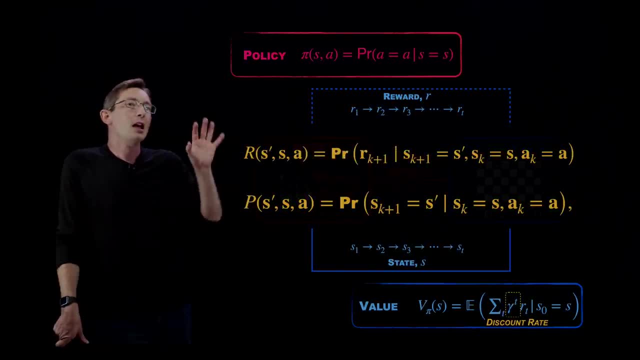 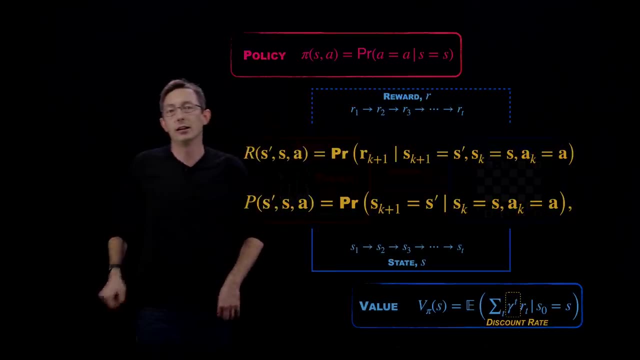 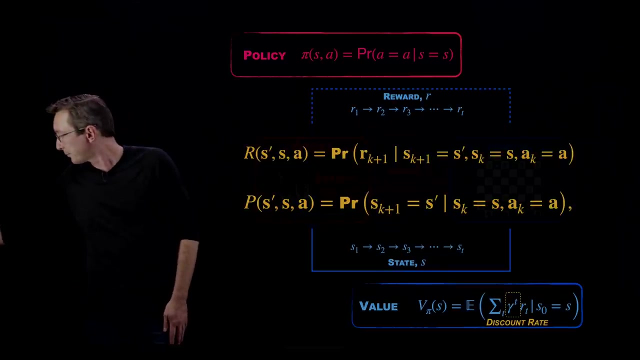 given a current, you know like, given a future state. And so this is the information we have at the outset and we're trying to learn an optimal policy and an optimal value function that kind of allow you to best play that game to maximize your future rewards. Good, And I'm going to walk through some 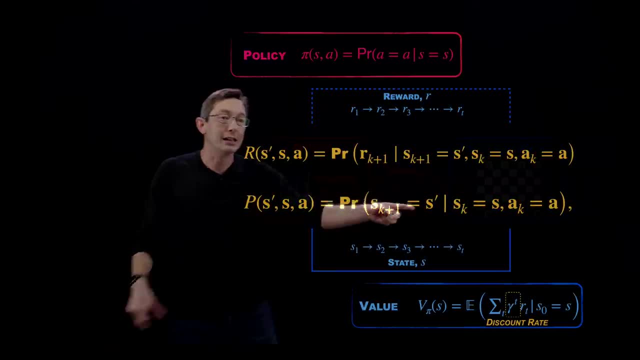 at the next time step will be S prime is some probability based on or conditioned on my state currently being S and my current action being A. So, given a current state S and a current action A, there is some probability that my system will. 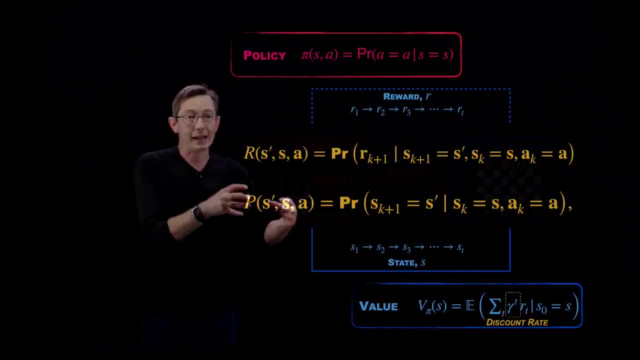 transition to a new state S prime and that's encapsulated in this probability model P. This is called a Markov decision process and it generalizes a normal Markov process to have some probability that the system will transition to a new state S prime. 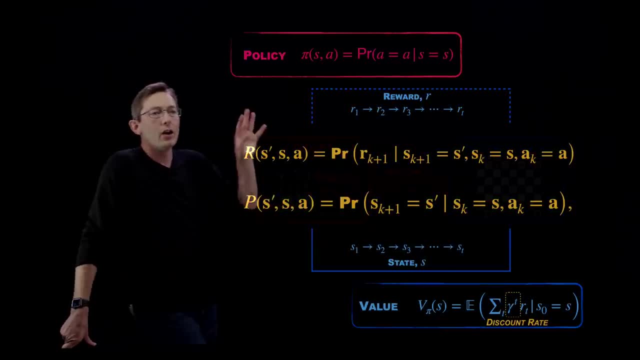 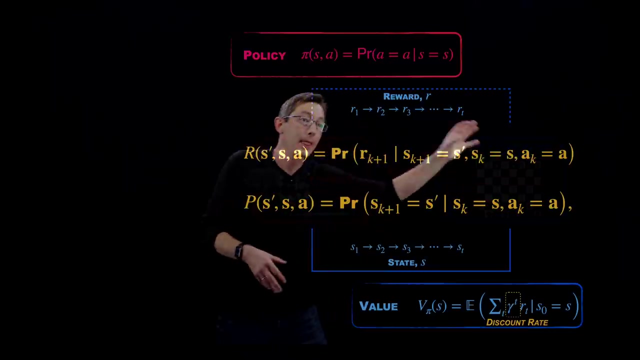 We also assume that we have some model of what the reward structure looks like. So what is the probability of a reward given some current state S or sorry, given a current state S and a current action A, and assuming that I move to a future state S prime in the next state? 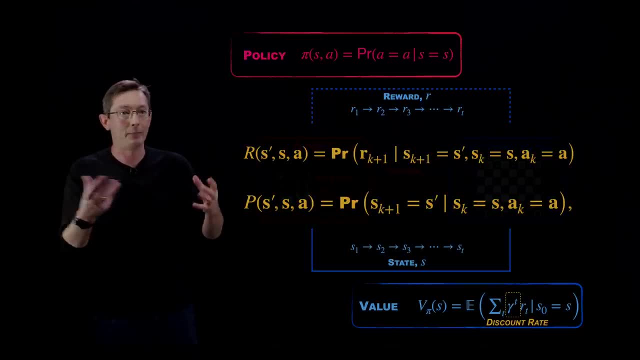 what is my expected reward given all of that happening? So, given kind of this information, what is my expected reward? What is my expected reward at the next time step? And again, this is kind of an assumption that you know the rules of the game you're playing. 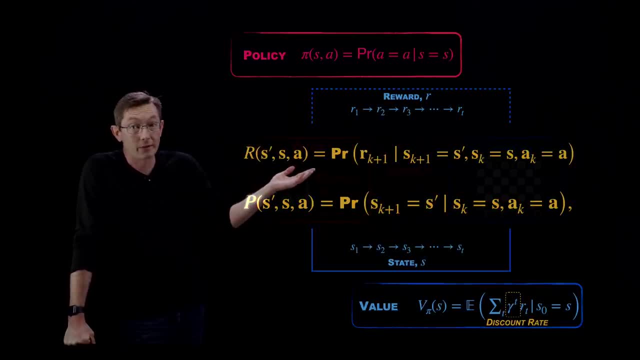 So if I'm playing chess, for example, the reward only comes at the very end of the game, but I know what the rules to win are. I know how to checkmate someone or how to not checkmate someone. You have to know that going in to play. And so this would basically say: 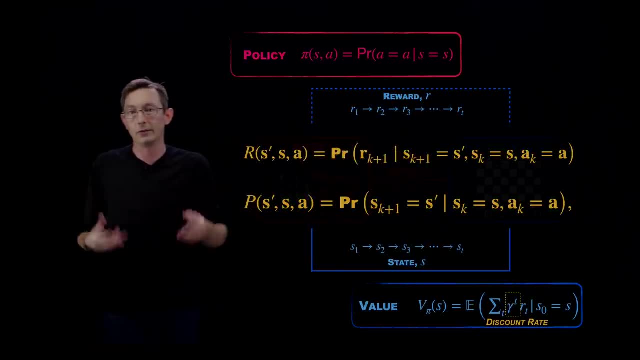 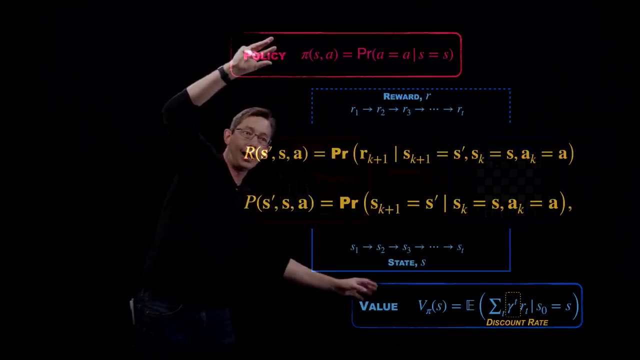 I know what my reward is- given a current like, given a future state, And so this is the information we have at the outset and we're trying to learn an optimal policy and an optimal value function that kind of allow you to best play that game to maximize your future rewards. 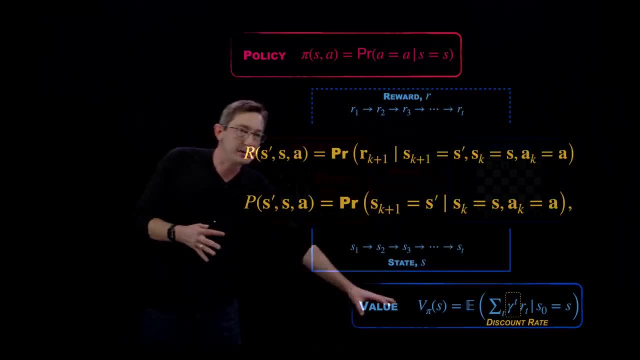 Good, And I'm going to walk through some properties of the value function that allow you to solve this problem. This seems like a big brute force problem. Let me take one step before I go into the value function. In the game of chess, for example, there are so many possible. 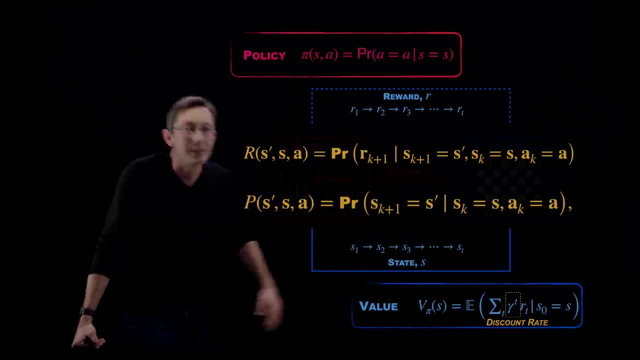 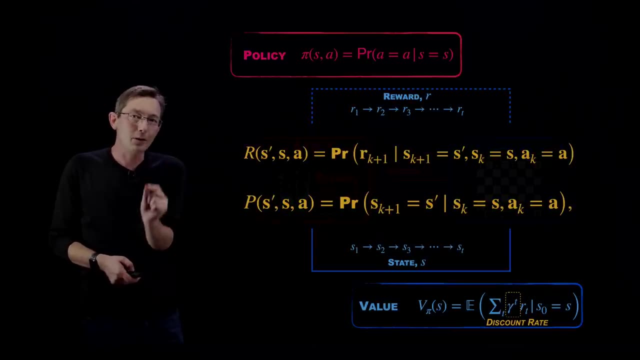 boards configurations, The state S. there are so many possible states that your chess board can be in something like you know: 10 to the 80. In fact, fun fact, the number of possible boards of chess that you can have is an unknown number. We know that it's very large, you know. 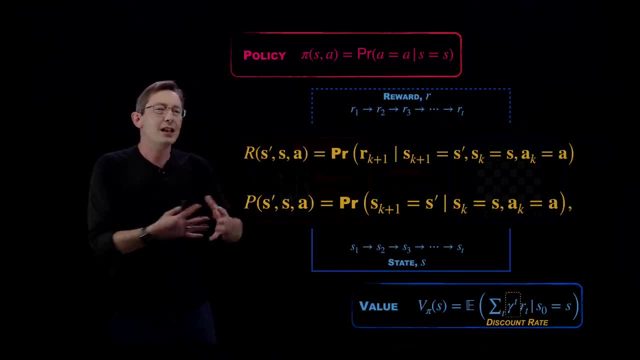 properties of the value function that allow you to solve this problem. This seems like a big brute force problem. Let me take one step before I go into the value function. In the game of chess, for example, there are so many possible boards configurations. The state S. 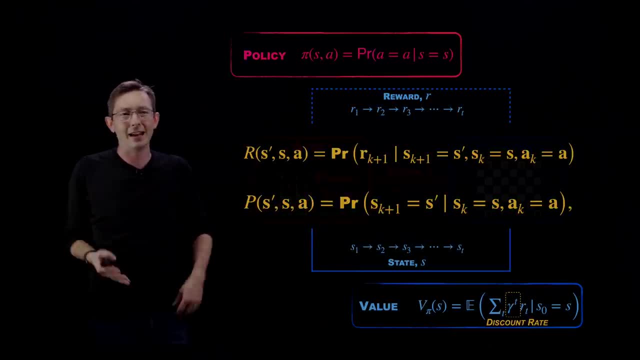 so many possible states that your chess board can be in something like you know 10 to the 80. in fact, fun fact, the number of possible boards of chess that you can have is an unknown number. we know that it's very large. you know 10 to the 80 or something on the order, but we don't know. 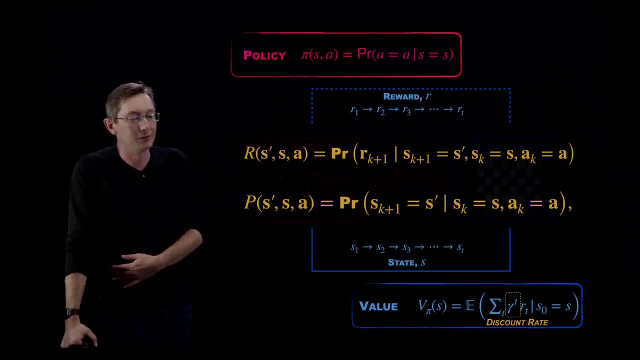 exactly what that number is, and i think that's kind of a fun fun fact that we know it's huge, but we can't actually perfectly quantify what that number is. it has someone famous's name, but but that's neither here nor there and so we can't actually compute this optimal value function. 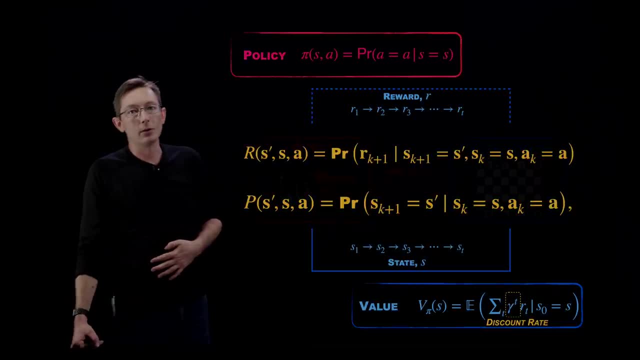 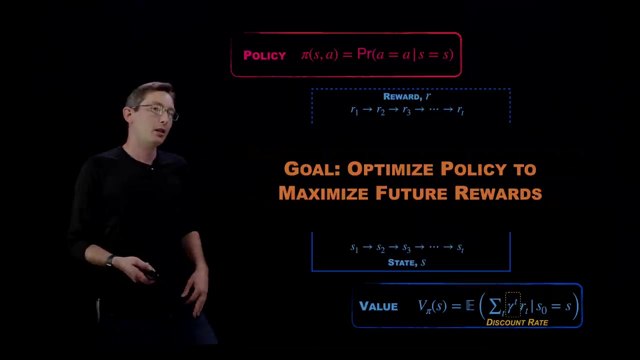 at all of those 10 to the 80 board conditions. so to solve for the optimal policy and to get this optimal value function would be a combinatorial, like brute force search over all possible states, and it just isn't even remotely feasible. okay, so we need some alternative and, uh, that that's what the dynamic 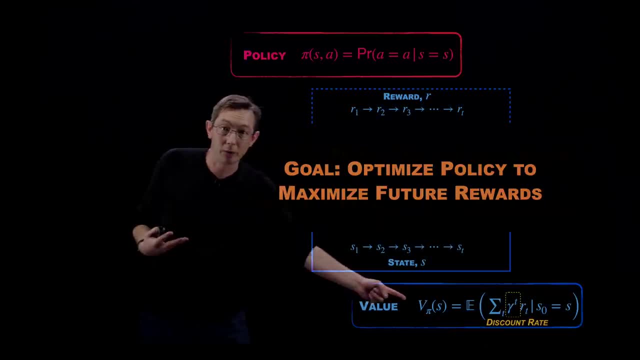 programming is going to allow us to do is to break this up into smaller sub problems so that i can think of, like, what's the optimal thing to do for three steps ahead, or for four steps ahead, or for five steps ahead. that's actually how you know. you've learned to play when you're a kid, is you? 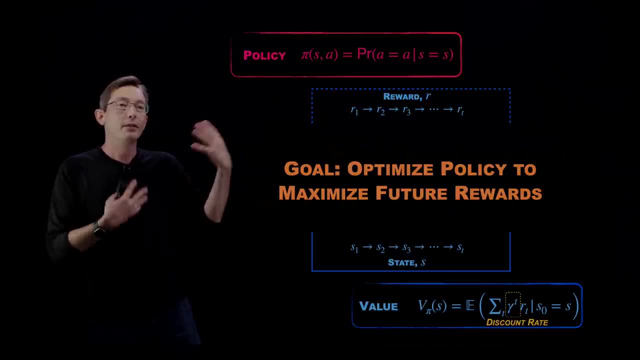 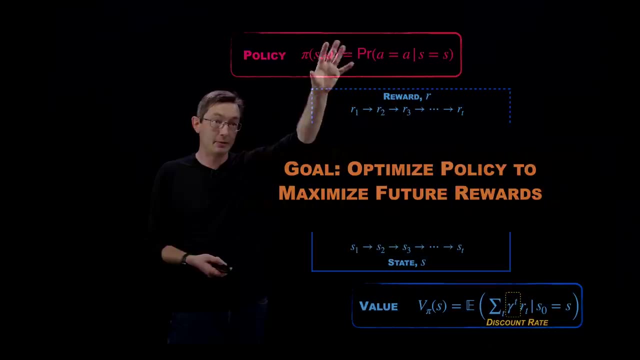 think a couple moves ahead and you optimize for that. that's what dynamic programming is going to allow us to do: break this up into smaller sub problems, okay, and so again, the goal is always to show that there are gonna be some things that you can do with basic performance design when you're 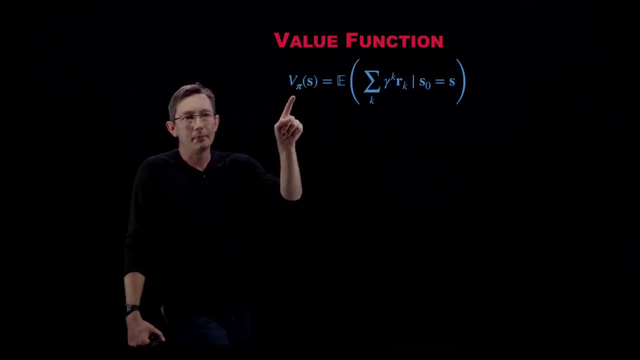 doing this. the real goal is for us to be able to look at how we do these things and we're going to go over those things through a more predictive way, using this project on how to do that in a sincere and logical way. and you think that's a simple proposal. that's a little bit more. 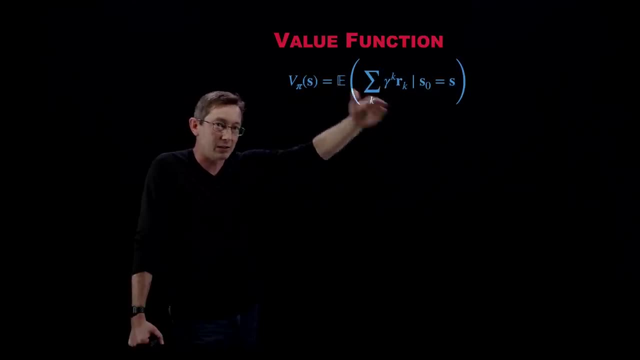 abstract, but it's a good idea for people to think about and then look at it when they're really thinking about putting together this basic model, to try and write something that's both a visual and a conceptual model, so that they can understand what the real goal is. if i think, 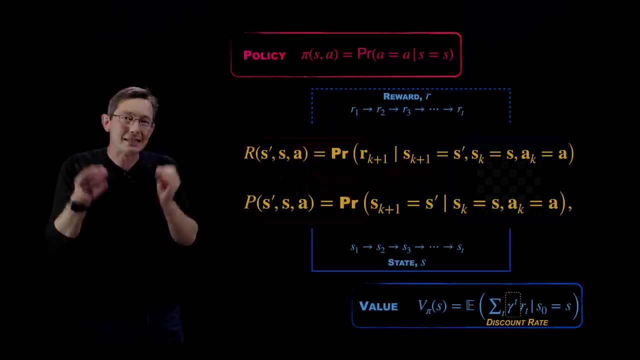 10 to the 80 or something on the order. but we don't know exactly what that number is, And I think that's kind of a fun, fun fact that we know it's huge, but we can't actually perfectly quantify what that number is. It has someone famous's name, but that's neither here nor there. 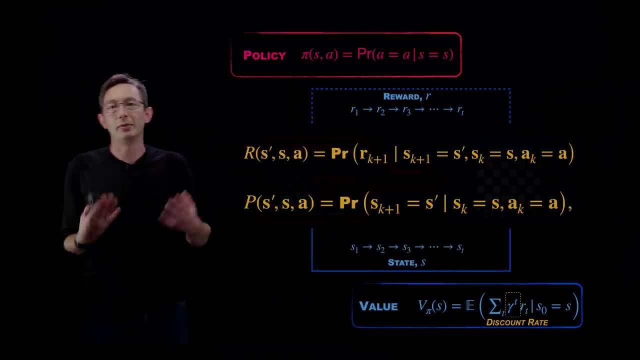 And so we can't actually compute this optimal value function at all of those 10 to the 80 board conditions. So to solve for the optimal policy and to get this optimal value function would be a combinatorial, like brute force search over all possible states, and it just isn't even remotely. 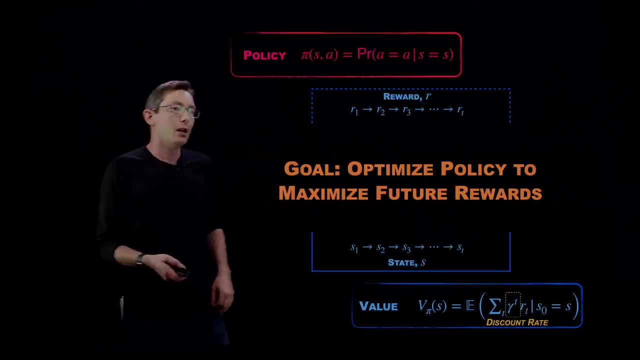 feasible, Okay, So we need some alternative, And that's what the dynamic programming is going to allow us to do- is to break this up into smaller sub-problems so that I can think of, like, what's the optimal thing to do for three steps ahead, or for four steps ahead, or for five steps ahead. That's actually. 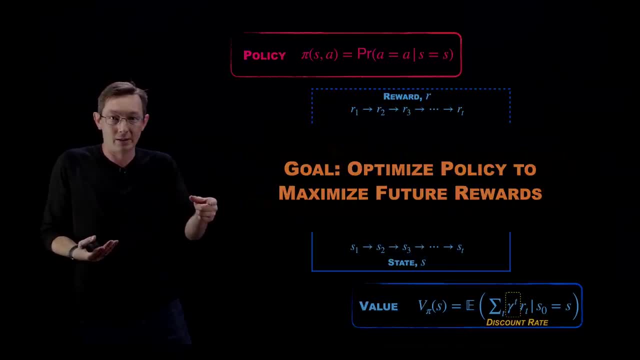 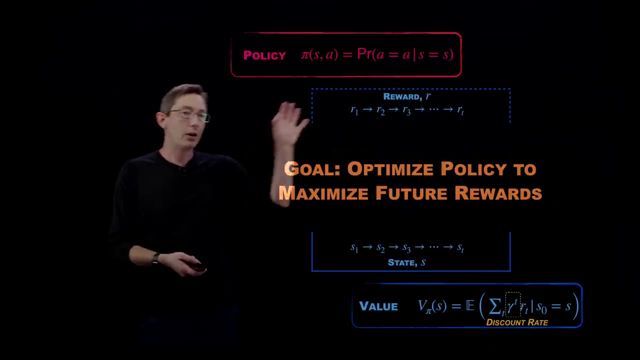 how you know you've learned to play when you're a kid is you think a couple moves ahead and you optimize for that. That's what dynamic programming is going to allow us to do: break this up into smaller sub-problems, Okay, And so again, the goal is always to optimize the policy. 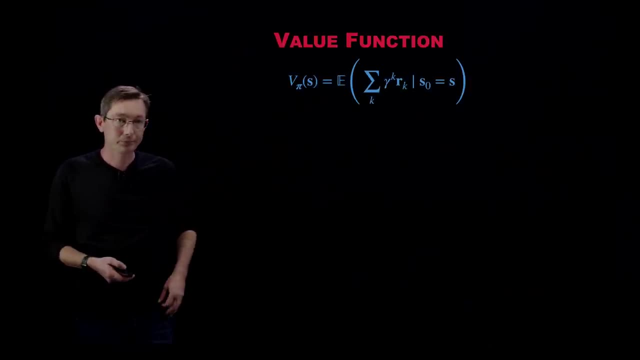 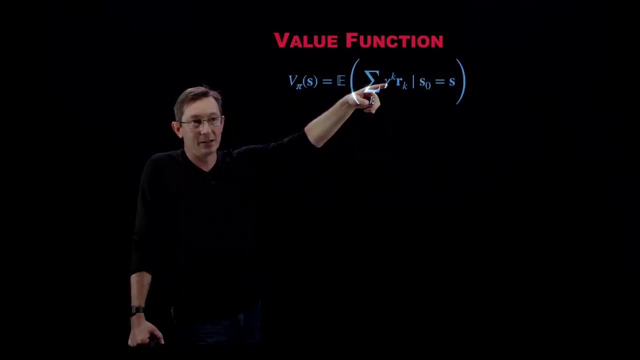 to maximize future rewards. That's all I can do as an agent. So we start with this value function. given some policy, pi, the value function at a given state. S is my expected future reward, discounted potentially by some gamma factor. So this gamma is a number between zero and one that discounts future rewards over current rewards. 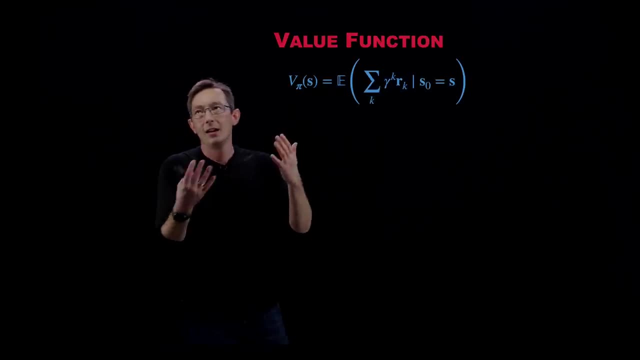 And that's kind of an economic principle. There's results that show certain optimality and convergence in this function. So it's really, really important that you think about these criteria for this kind of exponential decaying reward function. But that's what the value function does, is it? 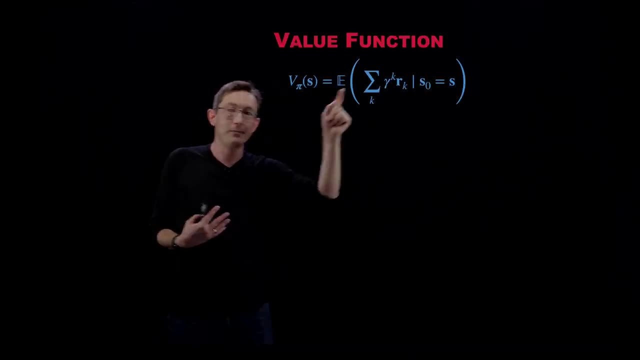 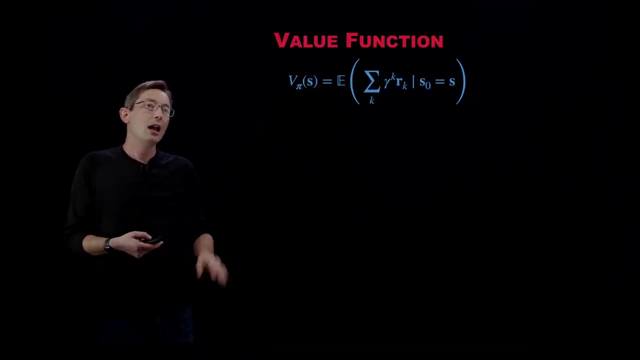 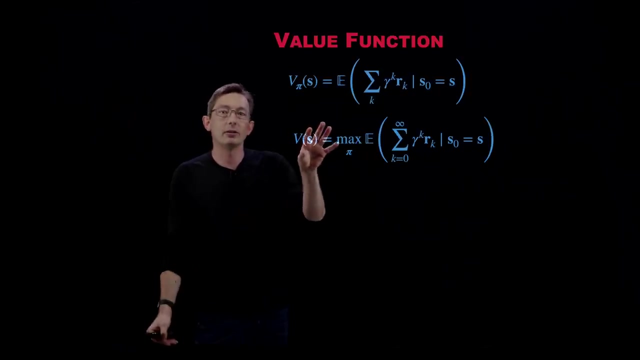 basically adds up your expected future reward, given that you're in a state S now and you know your first state is S and you enact an optimal policy pi. So it's kind of an implicit function of pi And if I drop the subscript pi, if I just talk about the value function, capital V. 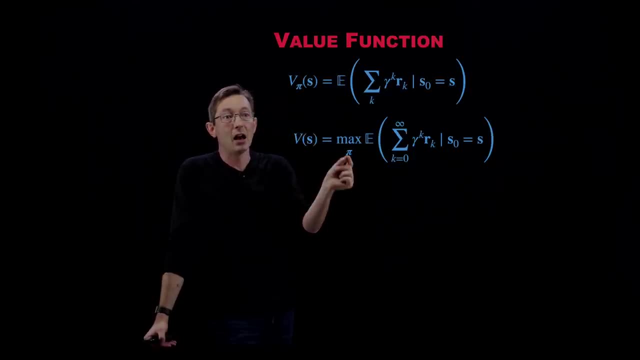 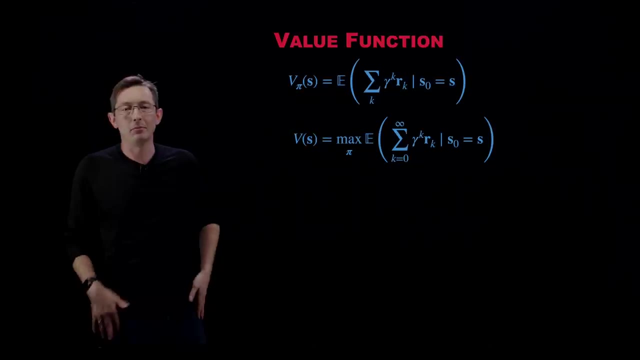 is the value of being in a state S assuming that I am working on the absolute best possible policy. Again, for any game that you can name, like chess or Go, like most games, you have no idea what this best policy is. 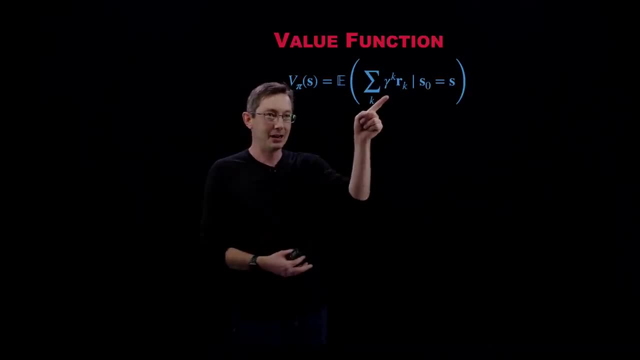 show certain optimality and convergence criteria for this kind of exponential decaying reward function. But that's what the value function does, is it basically adds up your expected future reward, given that you're in a state S now and your first state is S and you enact an optimal. 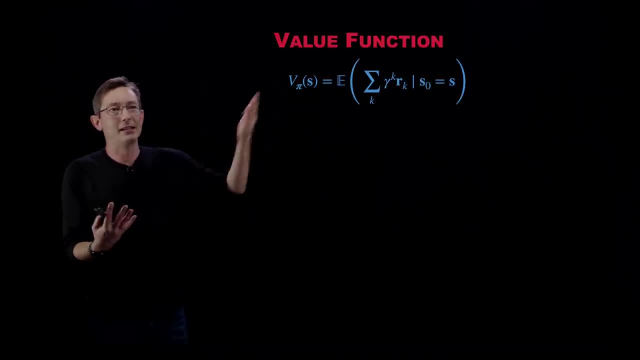 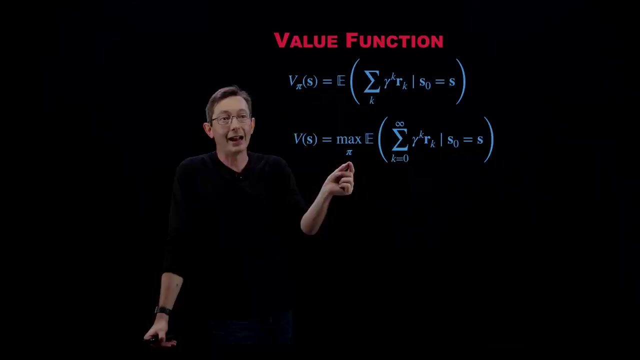 policy pi. So it's kind of an implicit function of pi. And if I drop the subscript pi, if I just talk about the value function, capital V, then this capital V value function is the value of being in a state S assuming that I am working on the absolute best possible policy, Again, for any 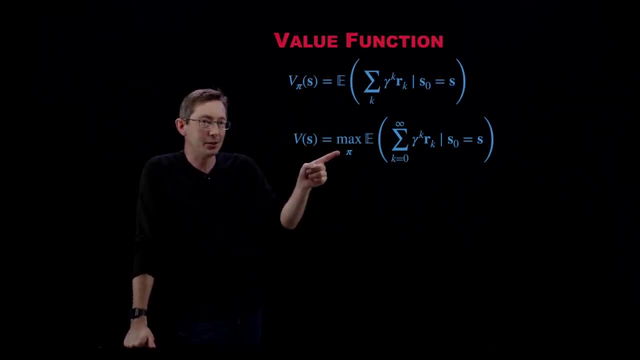 game that you can name like chess or go like most games. you have no idea what this best policy is, but there is some hypothetical best policy pi, and if you always played that best possible policy pi, this V would be the value. 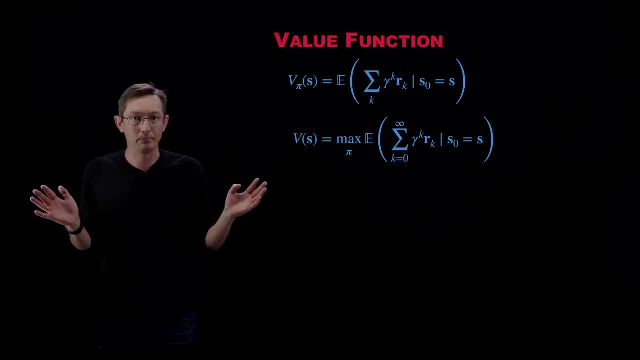 of being in a particular state, assuming you do the best thing possible. Good, And one of the really really cool things. so this is what Bellman figured out, Richard Bellman kind of. the rest was history. He figured this property out that allowed him. 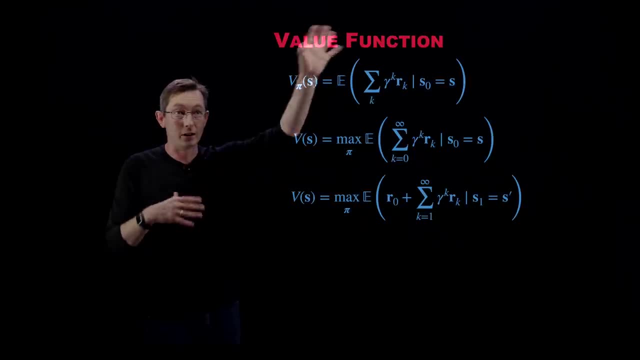 to invent dynamic programming and a large part of the field of reinforcement learning. So this value function here, this exact expression: you can take this sum of future rewards and break it up into the current reward at time step now. zero means now plus all of the future rewards. 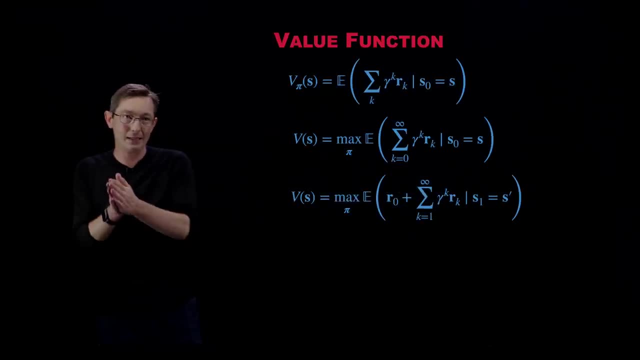 starting at time, step one to infinity. So I take my sum of all of my rewards at time now to infinity and I break that up into my reward now plus the sum of all of the rewards at the next state to infinity. So now this is the reward, given that my current state 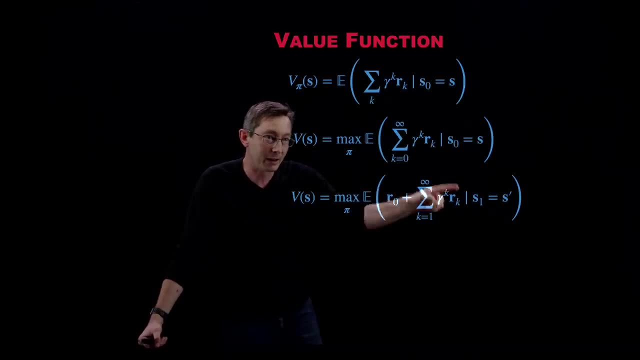 at time now, is F. This is my reward, given that my next state- S1, at the next time step- is S prime, And so what this allows you to do is essentially rewrite your value function. Your value function, given the best policy possible. 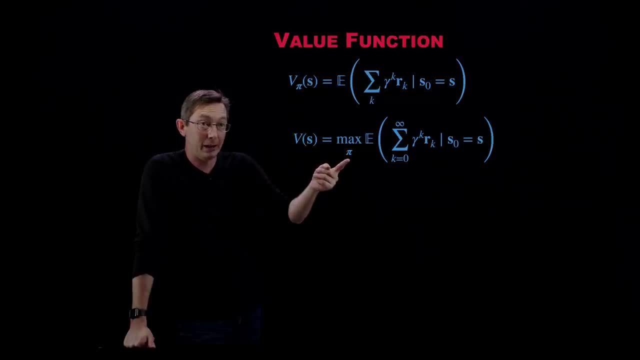 but there is some hypothetical best policy pi and if you always played that best possible policy pi, this V would be the value of being in a particular state, assuming you do the best thing possible. Good, And one of the really really cool things. 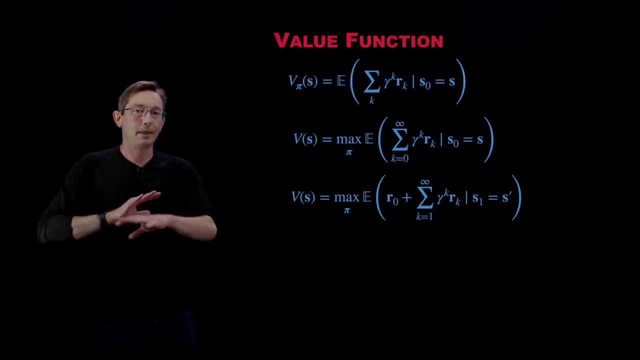 so this is what Bellman figured out. Richard Bellman kind of. the rest was history. He figured this property out that allowed him to invent dynamic programming and a large part of the field of reinforcement learning. So this value function here, this exact expression. 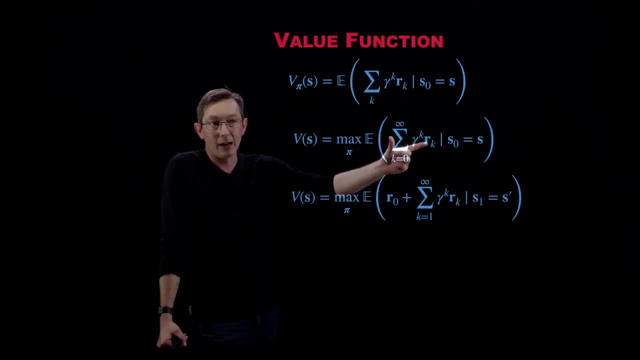 you can take this sum of future rewards and break it up into the current reward at time step now. zero means now plus all of the future rewards, starting at time step one to infinity. So I take my sum of all of my rewards at time now to infinity. 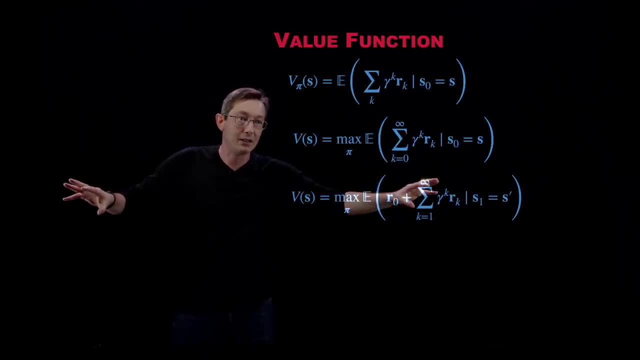 and I break that up into my reward now plus the sum of all of the rewards at the next state to infinity. So now this is the reward, given that my current state at time now is S. This is my reward, given that my next state 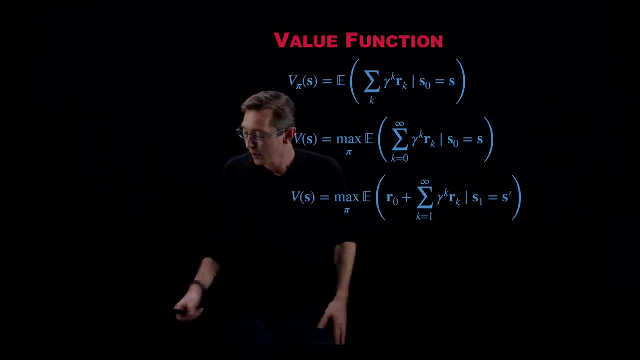 S. at the next time step is S' And so what this allows you to do is essentially rewrite your value function. Your value function, given the best policy possible, is whatever your current reward is, plus a discounted value function at this next state, S. 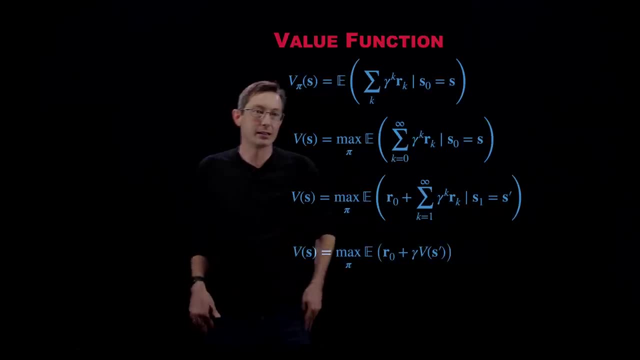 And so you can recursively define your value function like this: My value function at my current state is a function of S, the value function at my next state S' And that's really really powerful. So this means that if I do the absolute, 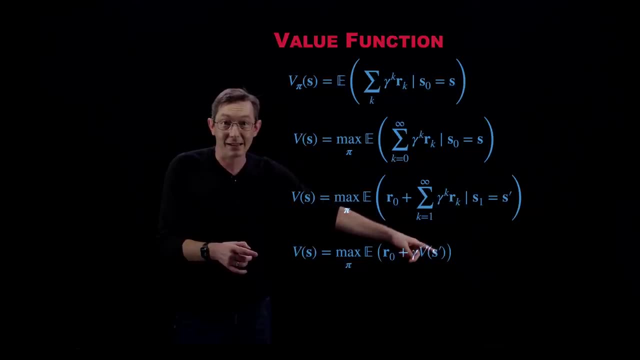 if I know what this value function is and I know what the best next state is, all I have to do is take an action now to get me to that next best state in the future, And so this is a recursive expression that allows you to break it up into sub-problems. 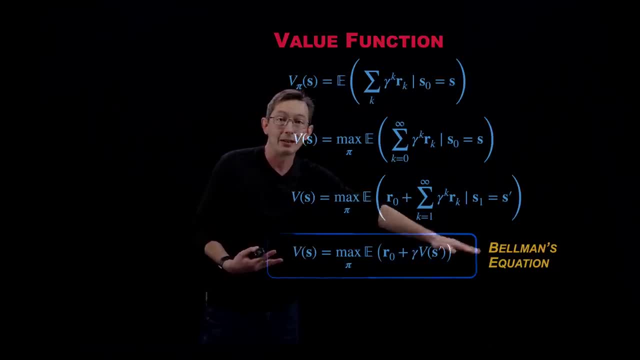 This is called Bellman's equation or Bellman's optimality condition. And if this is satisfied for a problem, if the value function, the thing you're trying to optimize, is a recursive function of itself, at the next time step you can break this problem up into sub-problems. 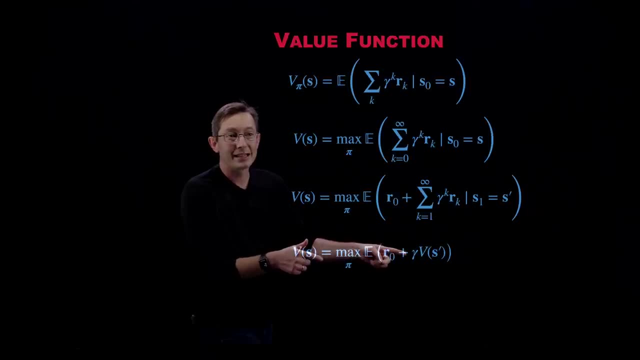 is, whatever your current reward is, plus a discounted value function at this next state S, And so you can recursively define your value function like this: My value function at my current state is a function of the value function at my next state S prime. 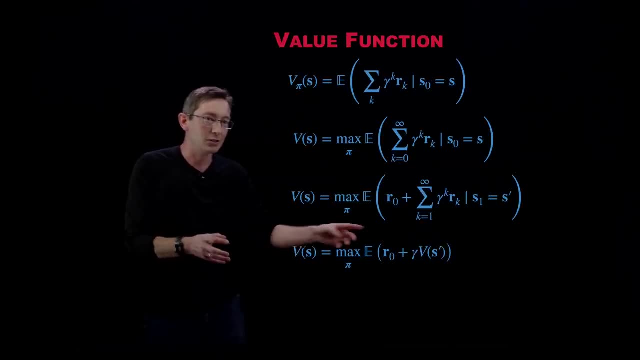 And that's really, really powerful. So this means that if I do the absolute, if I know what this value function is and I know what the best next state is, all I have to do is take an action now to get me to that next best state in the future. 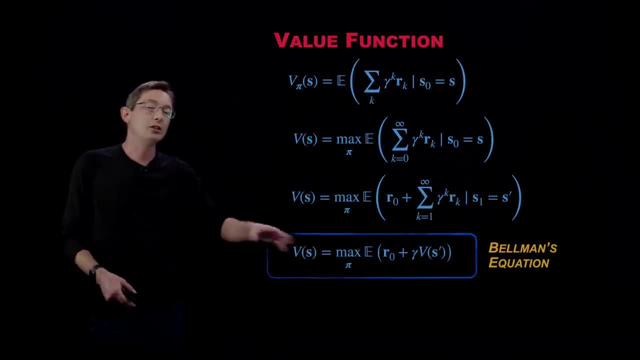 And so this is a recursive expression that allows you to break it up into sub-problems. This is called Bellman's equation or Bellman's optimality condition, And if this is satisfied for a problem, if the value function, the thing you're trying to optimize- 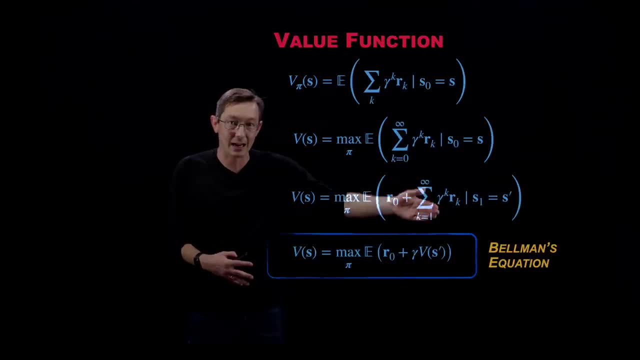 is a recursive function of itself. at the next time step, you can break this problem up into sub-problems, You can optimize locally and if you optimize locally enough in all of these different states and you put them together, you still have an optimal solution. 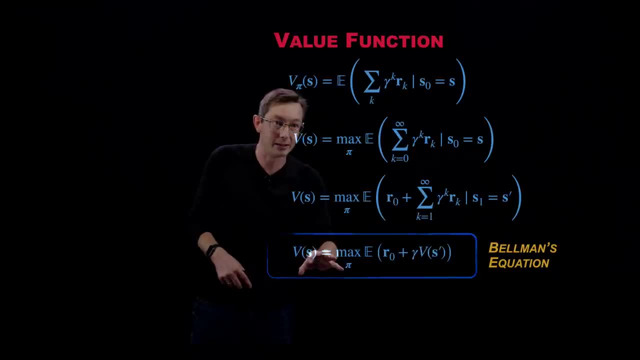 So, basically, I can optimize this sub-problem and then plug it into this problem and it's still optimal. That's really simple but very powerful, And once I have my optimal value function. so assuming that I just you know. 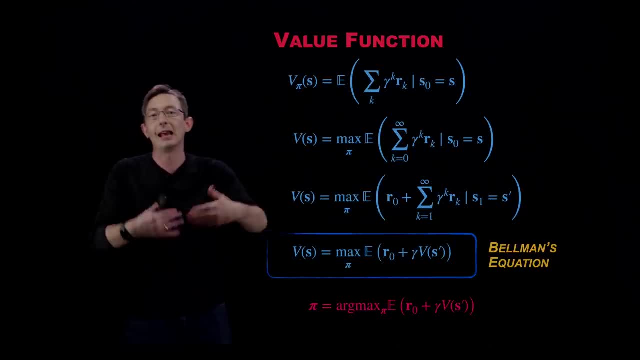 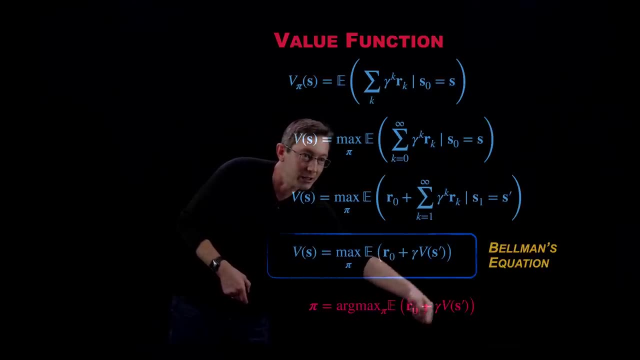 I did this and I had this optimal value function and maybe someone handed me an optimal value function. then I can always extract from this expression here this optimal value function. I can always extract the policy pi as the pi that maximizes. 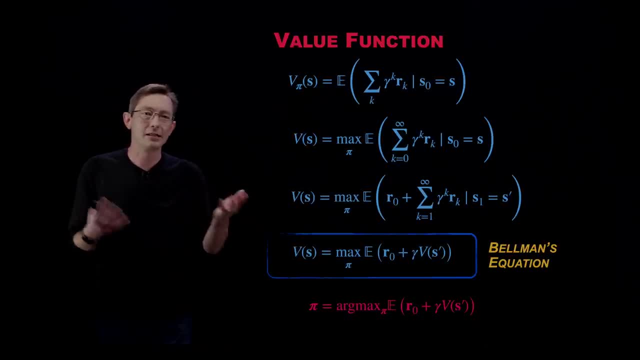 This expected reward. It's a little circular here. We're maximizing over the policy pi, this expression. Arg max means the pi that maximizes this expression. So you can always extract a policy from a value function. Okay, And given a policy, you can create a value function. 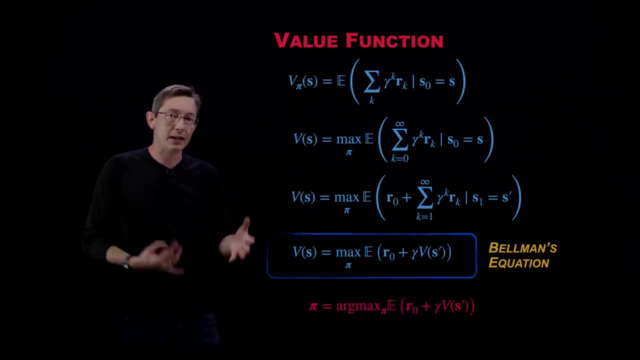 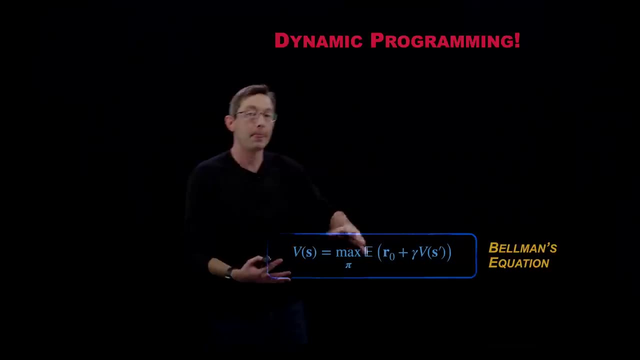 So this is Bellman's equation and this is the basis of dynamic programming. So dynamic programming is how we solve, how we we build, how we build up this value function. Again, we assume we know the rules of the game. 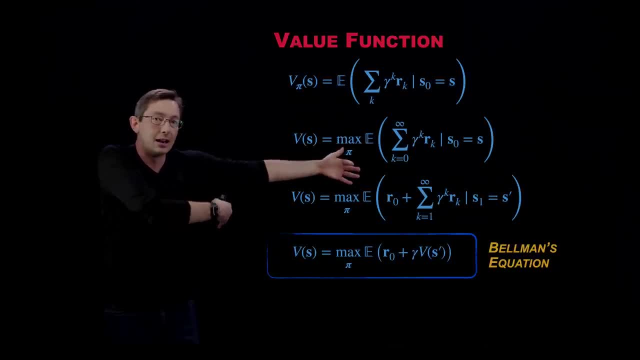 You can optimize locally And if you optimize locally enough at all of these different states and you put them together, you still have an optimal solution. So, basically, I can optimize this sub-problem and then plug it into this problem and it's still optimal. 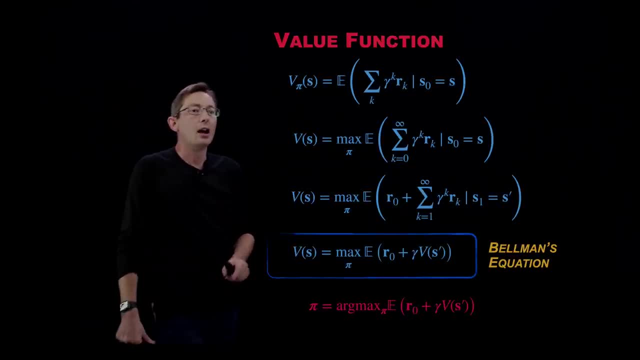 That's really simple but very powerful. And once I have my optimal value function- so assuming that I just you know I did this and I had this optimal value function and maybe someone handed me an optimal value function- then I can always extract from this expression here. 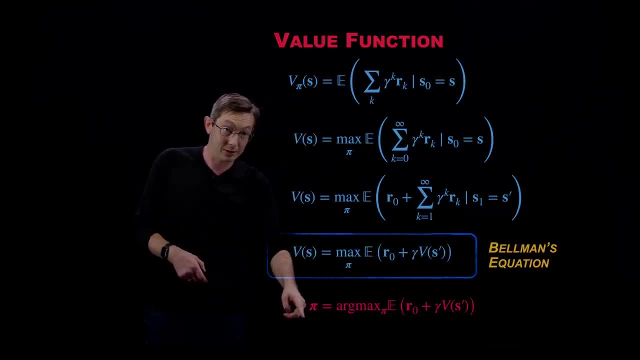 this optimal value function, I can always extract the policy pi as the pi that maximizes this expected reward. It's a little circular here. We're maximizing this, we're maximizing over the policy pi. this expression, Arg max means the pi that maximizes this expression. 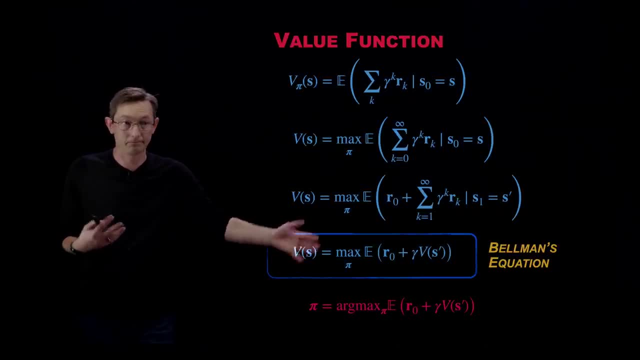 So you can always extract a policy from a value function. Okay, and given a policy, you can create a value function. So this is Bellman's equation and this is the basis of dynamic programming. So dynamic programming is how we solve. 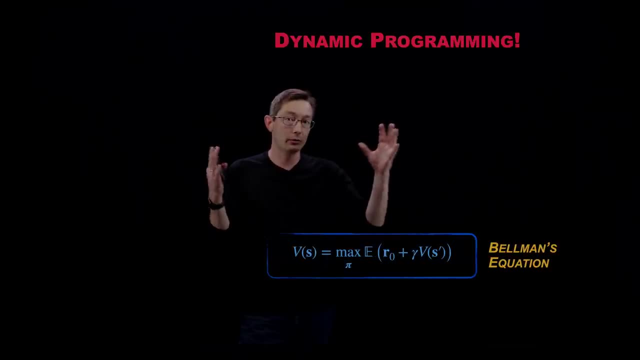 how we build up this value function. Again, we assume we know the rules of the game, but we don't know the value function or the optimal policy, pi. And so we can build this up, even for complex games using dynamic programming, as long as this equation is true, 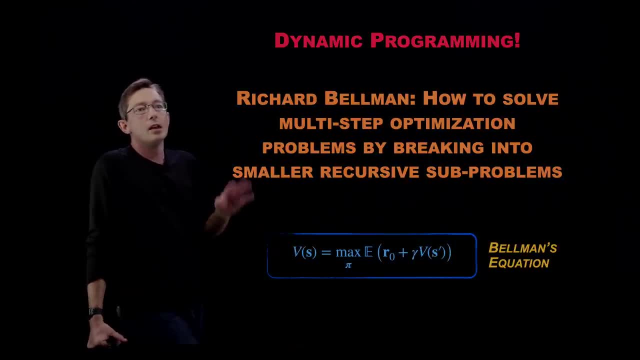 And it's true for Markov decision processes. So what Richard Bellman said is essentially: given systems that are recursive sub-problems like this, you can break them up, this multi-step optimization problem like how do I make a sequence of chess moves to win a game? 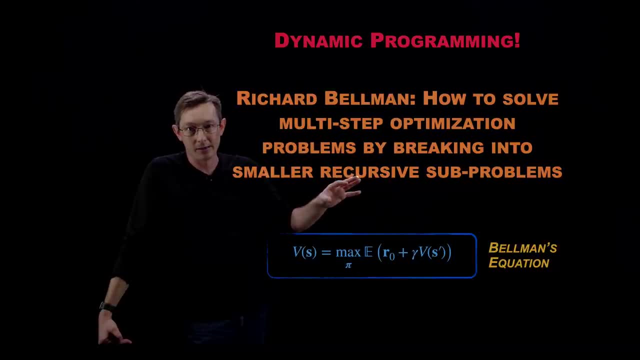 I can break that up into a number of steps, break them into smaller, algunas of significant sub-problems and then, when I can track it out, I can refer that in, in a space that is very tiny, to a number of smaller sub-problems. 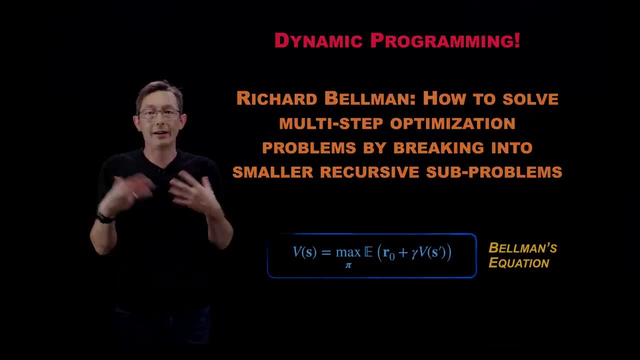 where, if I optimize over those sub-problems and then I put them all together, I still have an optimal action policy. And there's a lot of details of dynamic programming, kind of how you program this up in a computer, how you actually do this. 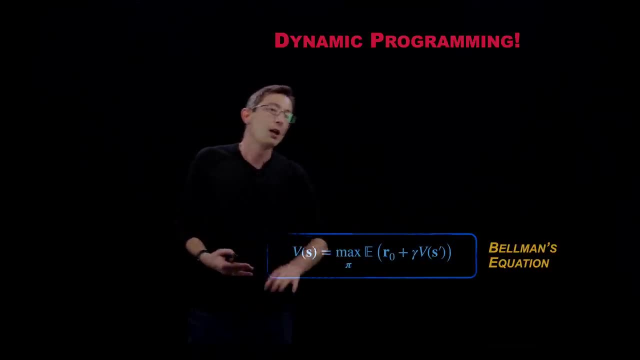 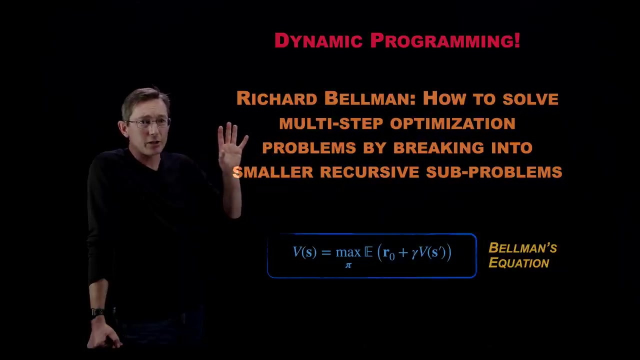 but we don't know the value function or the optimal policy pi, And so we can build this up even for complex games using dynamic programming, as long as this equation is true, And it's true for Markov decision processes. So what Richard Bellman said is essentially: 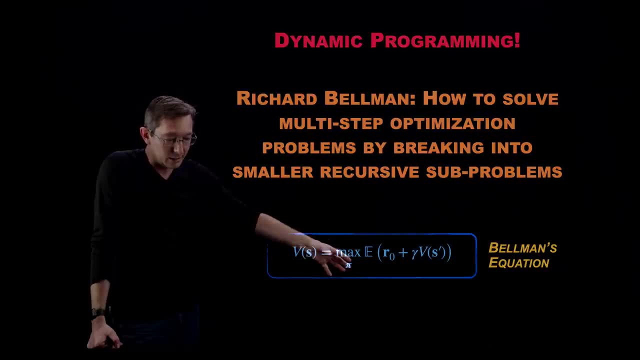 given systems that are recursive sub-problems like this, you can break them up. this multi-step optimization problem, like how do I make a sequence of chess moves to win a game- I can break that up into a number of smaller sub-problems. 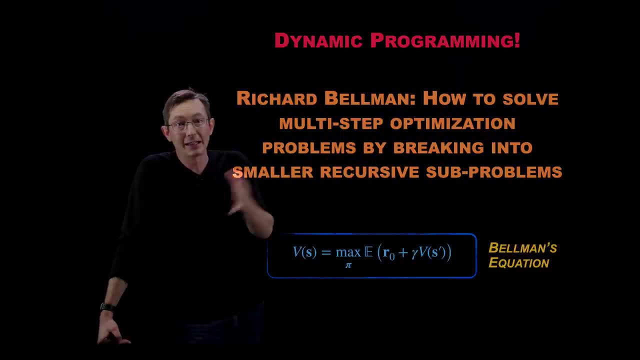 where, if I optimize over those sub-problems and then I put them all together, I still have an optimal action policy. And there, you know, there's a lot of details of dynamic programming, kind of how you program this up in a computer. 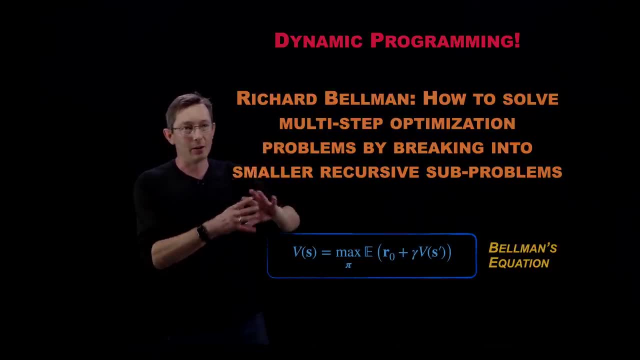 how you actually do this. Maybe that'll be, you know, a detailed lecture for another day. There are kind of two big approaches to dynamic programming. There are kind of two big approaches to dynamic programming. There are kind of two big approaches to dynamic programming. 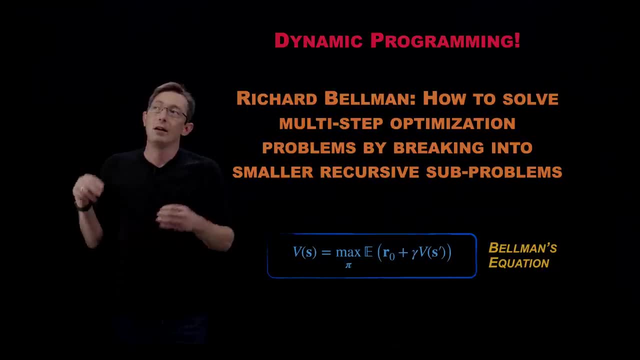 There is the top-down approach and the bottom-up approach, And so in the top-down approach you essentially list out all possible sub-problems. You kind of list out all possible little sub-problems and you try to solve all of them. 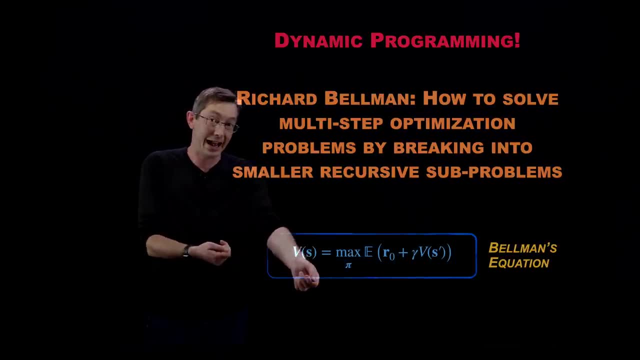 And you basically just keep track. Every time you need a sub-problem, you see if it has been solved. If so, you use it, If not, you solve it And recursively you end up filling out this table of sub-problems until eventually you've kind of brute force. 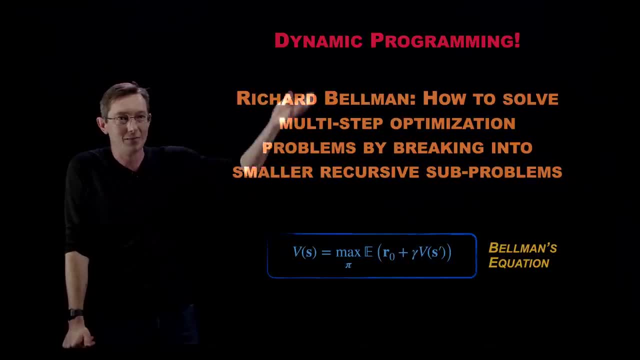 solved the whole thing. I'll point out you can't solve chess using dynamic programming. It's too big. You have to use other approximate methods, things like deep learning and things like that. But it's a good cartoon. You can solve tic-tac-toe using dynamic programming. 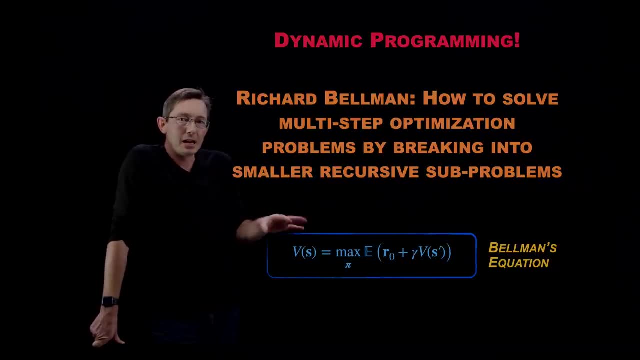 That's one of my homework exercises. So the top-down approach is basically to create this table or memoization of all sub-problems and solve them as needed until they're all solved. The bottom-up approach is basically to always start with the smallest sub-problems and work your way back. 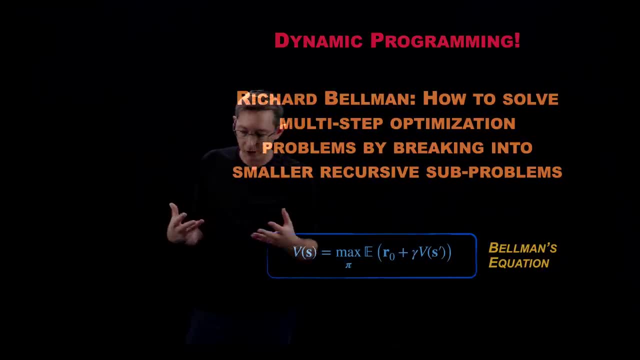 Maybe that'll be a detailed lecture for another day. top-down approach: you essentially list out all possible sub problems. you kind of list out all possible little sub problems and you try to solve all of them and you basically just keep track. every time you need a sub problem, you see if it has been solved. if so, you use it. if not, you solve. 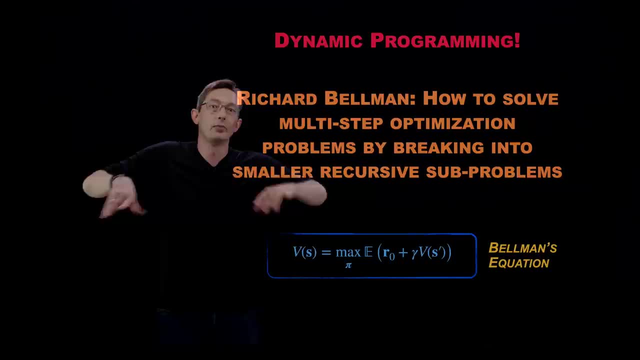 it and recursively you end up filling out this table of sub problems until eventually you've kind of brute force solved the whole thing. i'll point out: you can't solve chess using dynamic programming. it's too big. you have to use other approximate methods, things like deep learning. 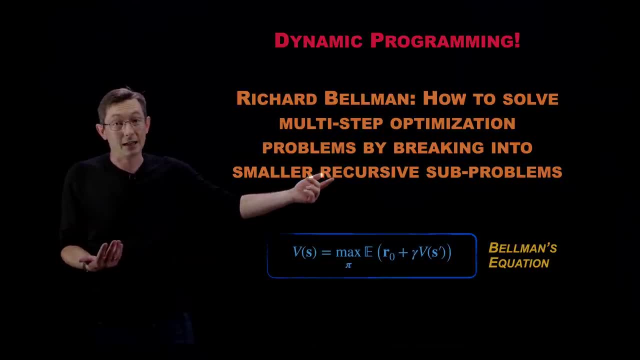 and things like that, but it's. it's a good cartoon. you can solve tic-tac-toe using dynamic programming. that's one of my homework exercises. so the top-down approach is basically to create this table or memoization of all sub problems and solve them as needed until they're all solved. 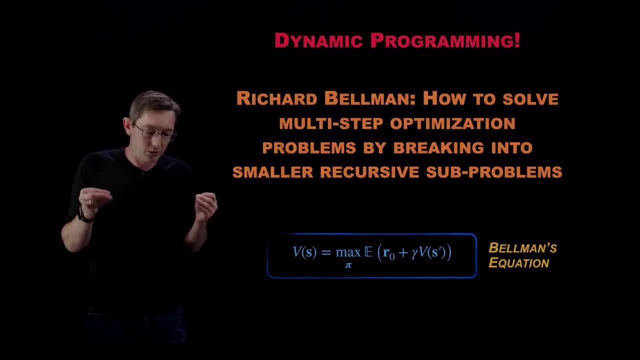 the bottom-up approach is basically to all always start with the smallest sub problems and work your way back, aggregating them into bigger problems. so the way you would think about that is you would start from every winning configuration, every configuration where you definitely got a reward and won, and then you'd 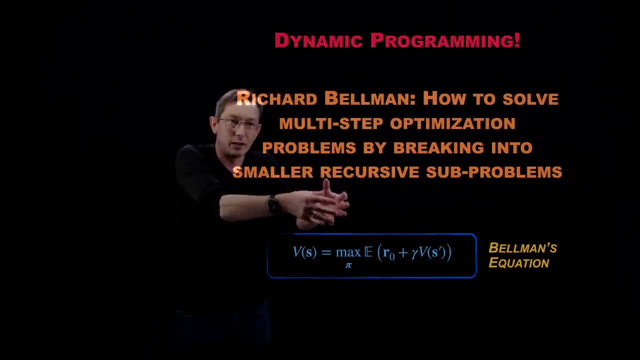 optimize one step back- what was the best move to get me in that position? and then you'd optimize two steps back- what was the best move, given that i want to be here- to get me in that position? and you'd kind of recursively build up bigger and bigger optimization sequence from from these. 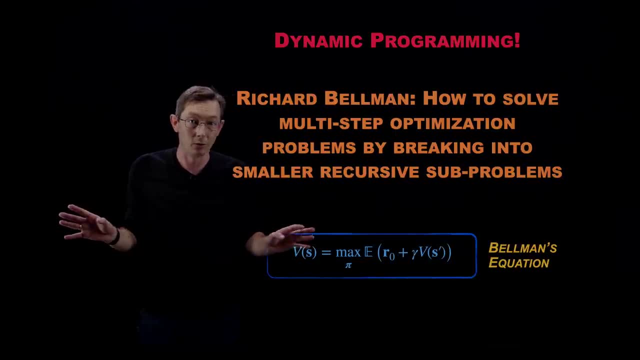 winning configurations or from locations where you know you're getting a reward. this is a massive simplification, but that's the basic idea of dynamic programming and although it's still very expensive and kind of a brute force approach, it's still better than a naive brute force approach. dynamic programming is really. 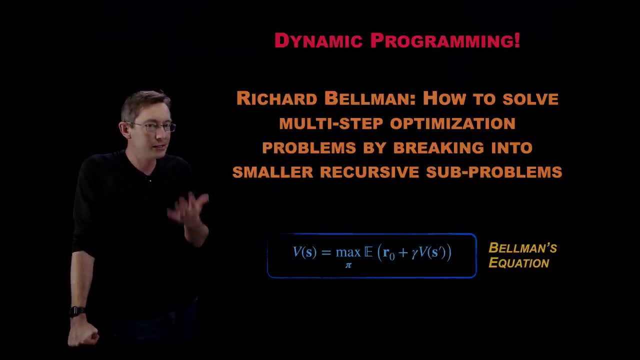 closely related. for those of you who are computer science people, it's closely related to divide and conquer methods, except that divide and conquer methods, like the quick sort algorithm, specifically rely on your problem being non-overlapping and non-recursive, whereas these are. this is a recursive optimization. 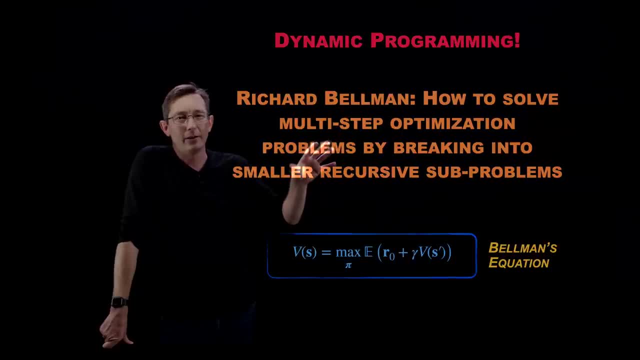 aggregating them into bigger problems. So the way you would think about that is you would start from every winning configuration, every configuration where you definitely got a reward and won, and then you'd optimize one step back. What was the best move to get me in that position? 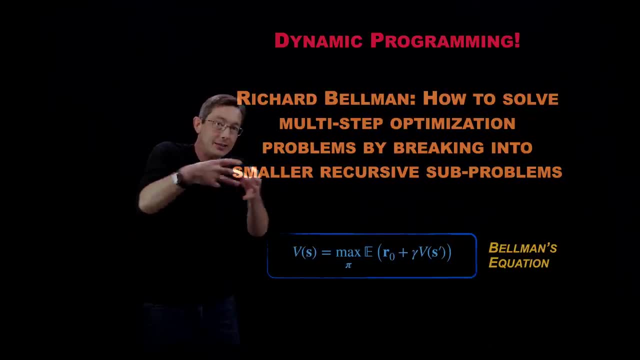 And then you'd optimize two steps back. What was the best move, given that I want to be here? What would I want to be here to get me in that position? And you'd kind of recursively build up bigger and bigger optimization sequence from these winning configurations. 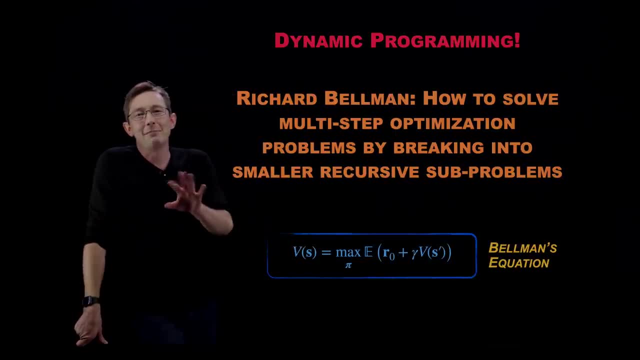 or from locations where you know you're getting a reward. This is a massive simplification, but that's the basic idea of dynamic programming And although it's still very expensive and kind of a brute force approach, it's still better than a naive brute force approach. 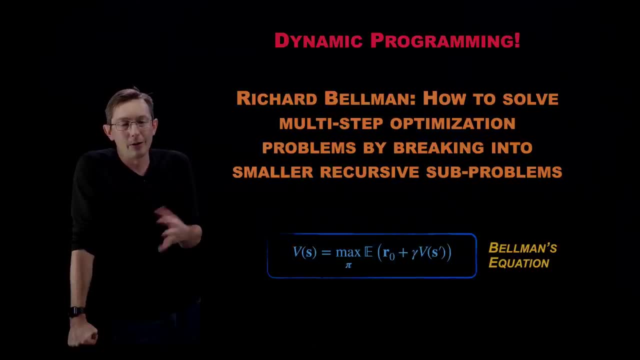 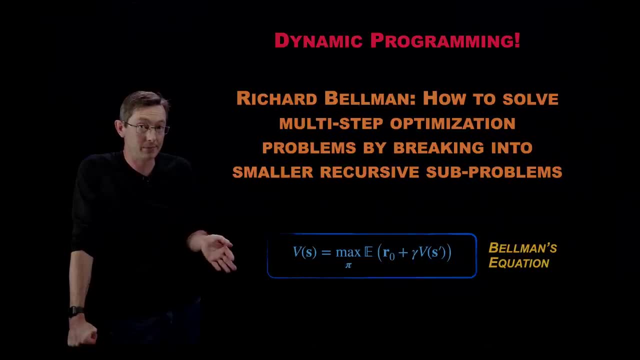 and you're a computer scientist, and you're a computer scientist and you're a computer scientist. it's closely related to divide and conquer methods, except that divide and conquer methods, like the quicksort algorithm, specifically rely on your problem being non-overlapping and non-recursive. 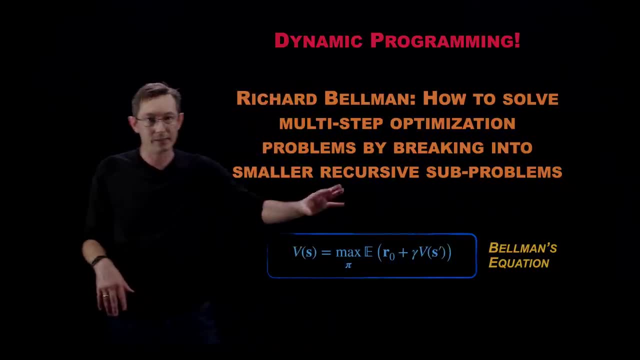 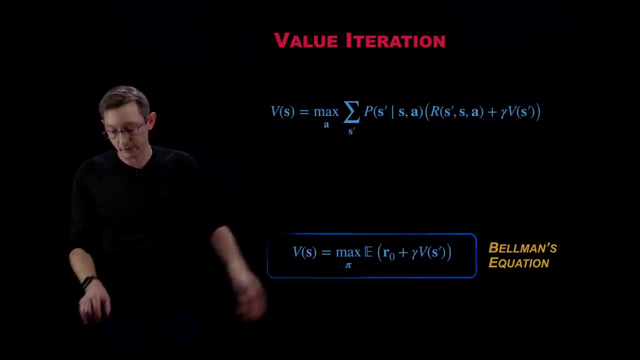 Whereas these are. this is a recursive optimization, So this is a bit more sophisticated. Okay, that was a lot, So now let's talk about how we actually do this, for value iteration, for example. So two of the leading algorithms that rely on dynamic programming. 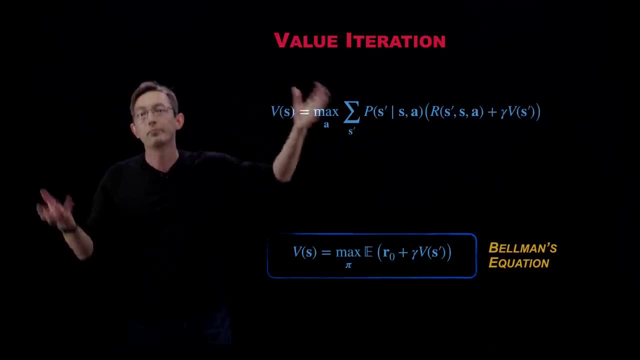 for model-based reinforcement learning are value iteration and policy iteration, And so value iteration is essentially going to allow me to use Bellman's optimality condition to iteratively build a refined estimate of my value function through trial and error, Not through trial and error. 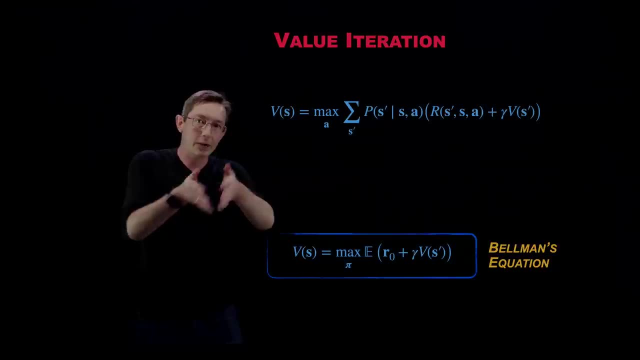 through optimizing a sequence of events through a known model, And there's ways of tweaking this so that you can do it through trial and error. That's called approximate dynamic programming And I'll talk about that later. So the idea is that the value function again. 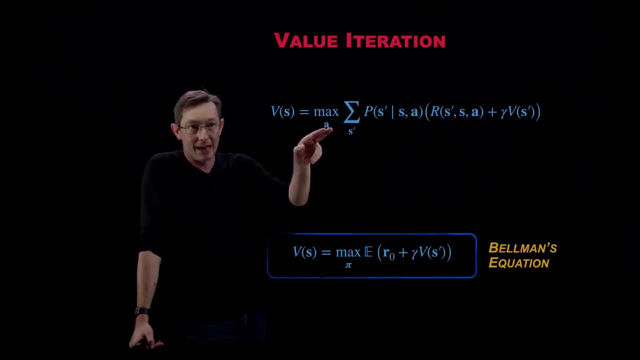 we're trying to maximize over the best, all of the possible actions. we're maximizing that action to give this optimal future reward. And so it's my reward now, plus a discounted value function at the next step in my model, given that action A. 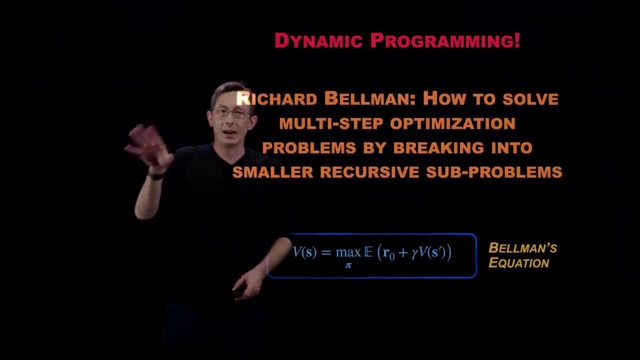 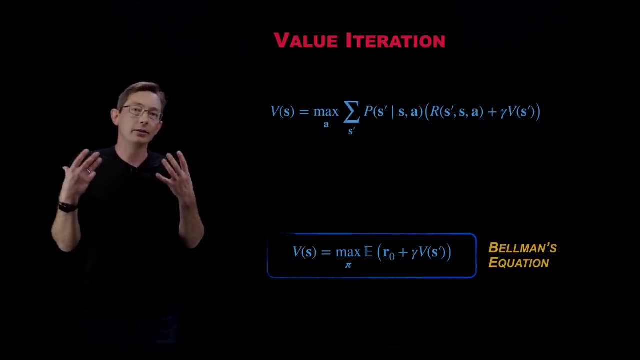 so this is a bit more sophisticated. okay, that was a lot, so now let's talk about how we actually do this. uh, for value iteration, for example. so two of the the leading algorithms that rely on dynamic programming for model-based reinforcement learning are value iteration and policy iteration, and so value iteration is essentially going to allow me to use bellman's 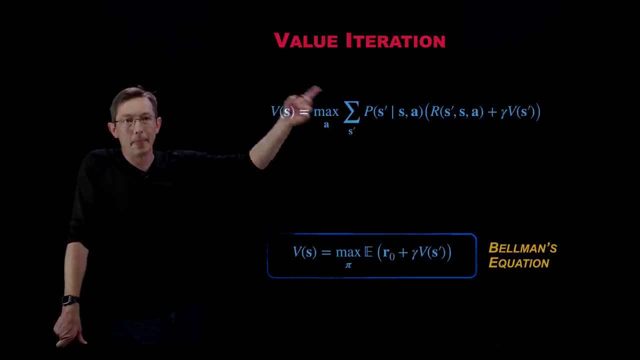 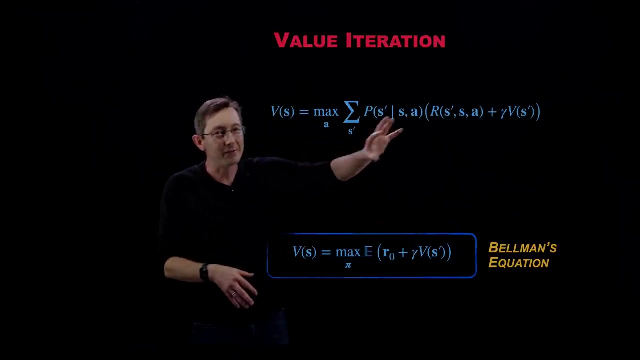 uh optimality condition to iteratively build a refined estimate of my value function through trial and error, not through trial and error through optimizing a sequence of events through a known model, and there's ways of tweaking this so that you can do it through trial and error. 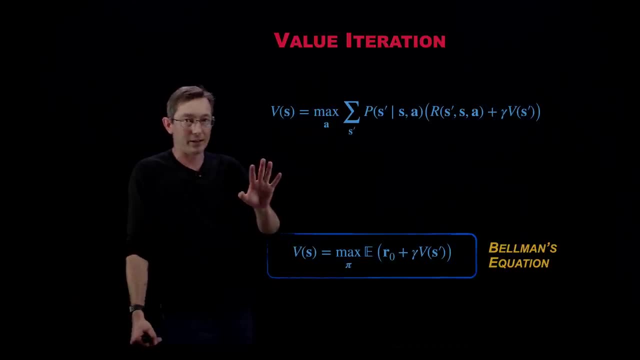 that's called approximate dynamic programming and I'll talk about that later. So the idea is that the value function. again we're trying to maximize over the best all of the possible actions. we're maximizing that action to give this optimal future reward. 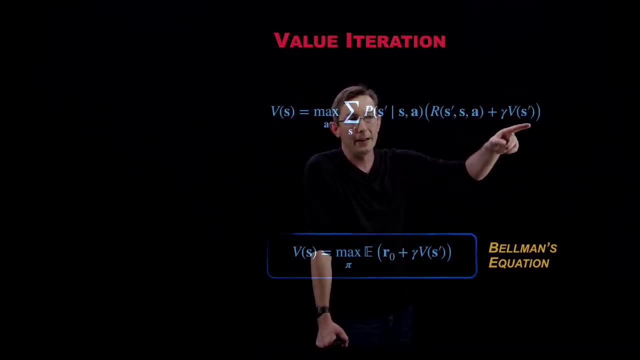 And so it's my reward now, plus a discounted value function at the next step in my model, given that action A And I have to sum up over these probabilities because this is a Markov decision process. So if this was a deterministic process, 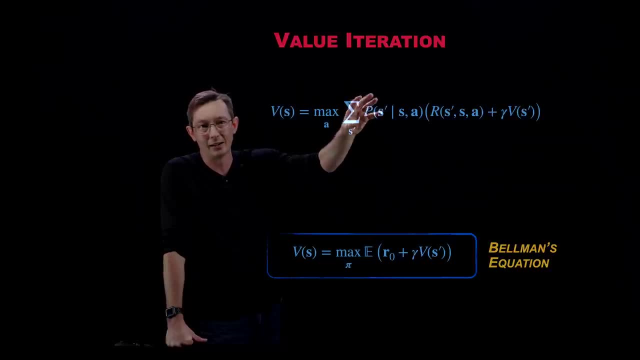 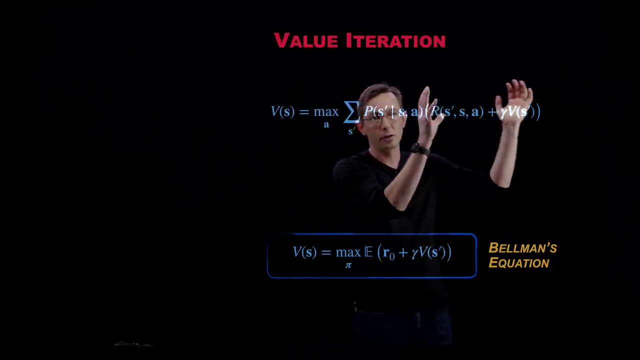 you wouldn't have this sum and this probability. but this is essentially necessary because this is a probabilistic Markov process. But this is the thing we're trying to maximize over, is our future total reward, which is my reward now, given this action I'm about to take. 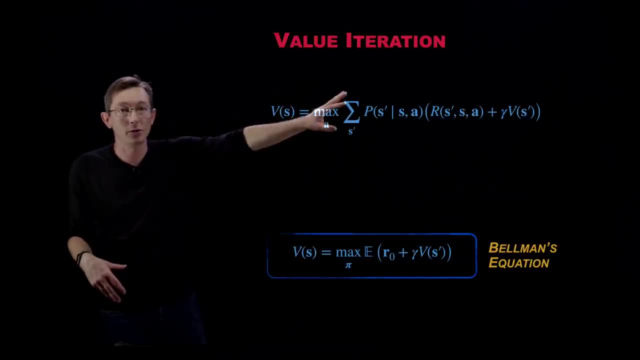 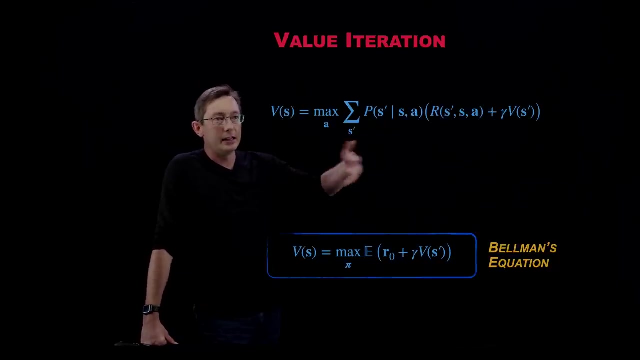 and my future value function. the sum of all my future rewards discounted by gamma. That's just. this is literally just this here rewritten, And so what we're essentially going to do is kind of iteratively start to update this V given this situation. 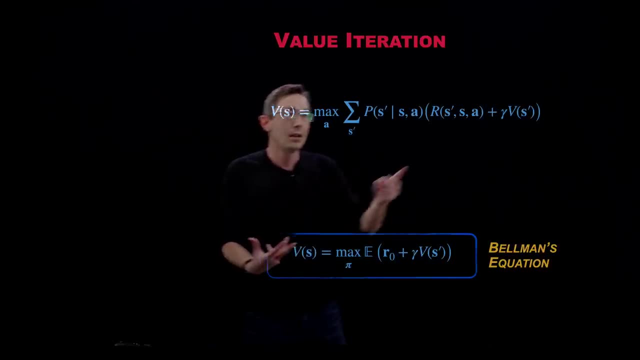 So we're going to in every sub problem, assuming that I have. this assumes two things: It assumes that I know the model of where I will be given an action from my current state And it assumes that I know V at my next state. 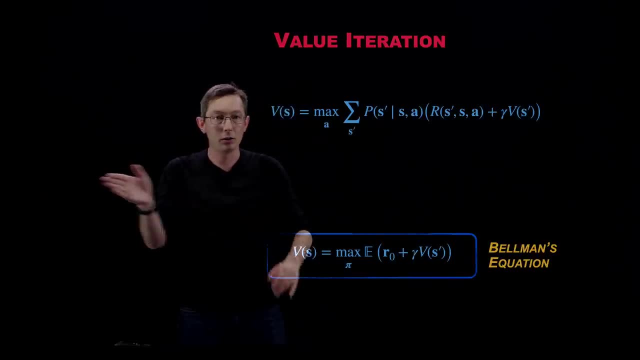 So I basically create a big table of my value function at all of the possible states And I might initialize it at zero or random or whatever. And then what I do is I started a state, So I'm initial, I randomly pick a state. 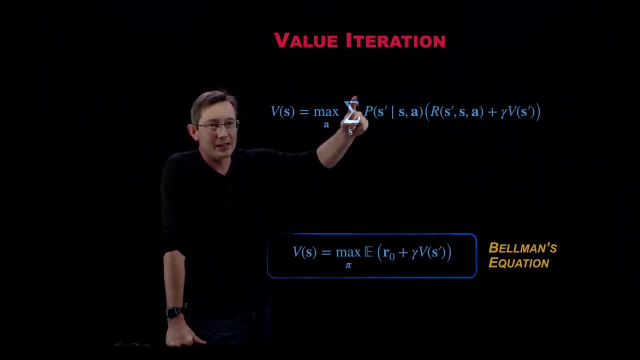 And I have to sum up over these probabilities- because this is a Markov decision process. So if this was a deterministic process, you wouldn't have this sum and this probability, but this is essentially necessary because this is a probabilistic Markov process. 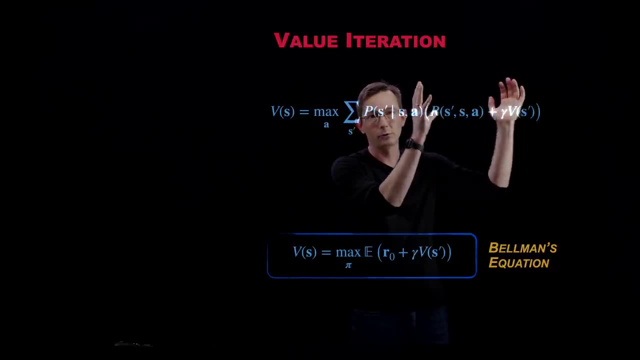 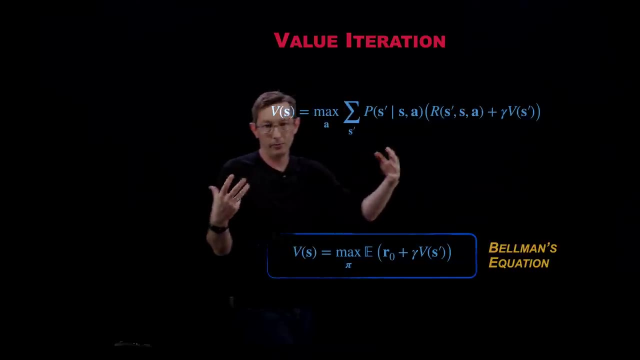 But this is the thing we're trying to maximize over is our future total reward, which is my reward now, given this action I'm about to take, and my future value function. the sum of all my future rewards discounted by gamma, That's just this, is literally just this, here rewritten. 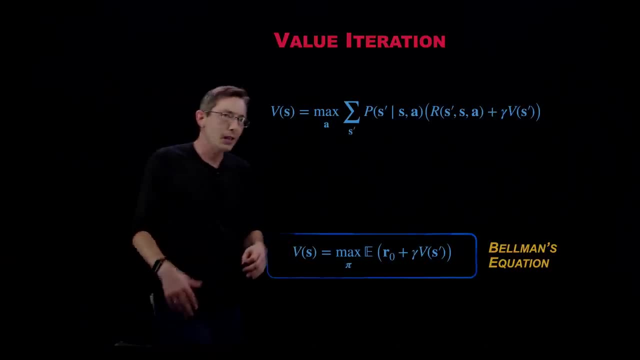 And so what we're essentially going to do is kind of iteratively start to update this V given this situation. So we're going to in every sub-problem, assuming that I have. this assumes two things. it assumes that I know the model. 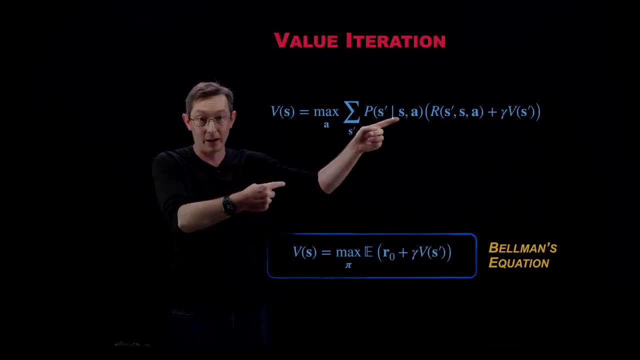 of where I will be given an action in my current state and it assumes that I know v at my next state. So I basically create a big table of my value function at all of the possible states and I might initialize it at zero or random or whatever. 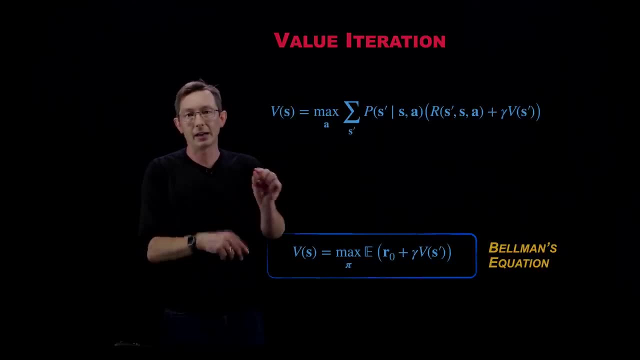 And then what I do is I start at a state, so I randomly pick a state, I start there and I start kind of playing the game. I start running through action sequences and updating my estimate of the value function. So let's see how this works. 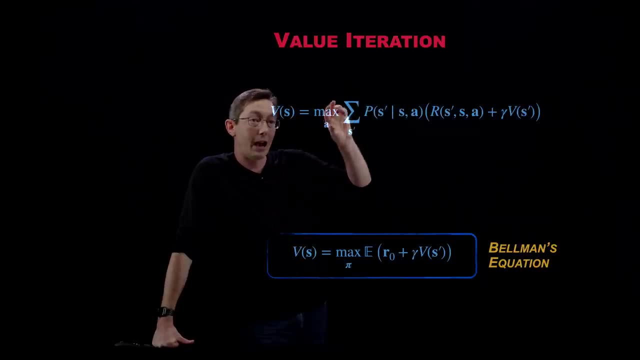 I'm in a state s now and what I'm going to do. I actually can evaluate this function for all actions because I know the reward function, I know the model p and I at least have a table of what I think the optimal value function is at all next states. 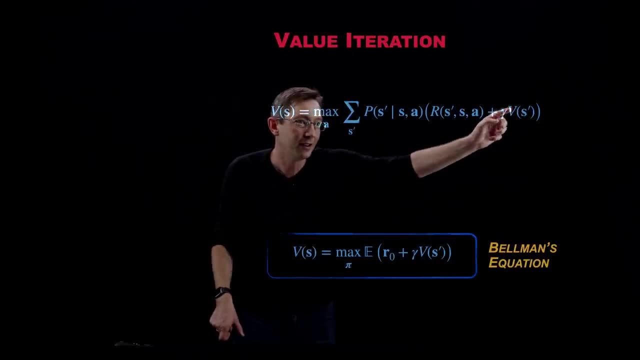 Now, that might be a really crummy estimate. This is kind of a v hat. This is an estimate of the value function. It might be a garbage estimate, but it's something. it's the best I've got, And so what I'm going to do is I'm going to maximize. 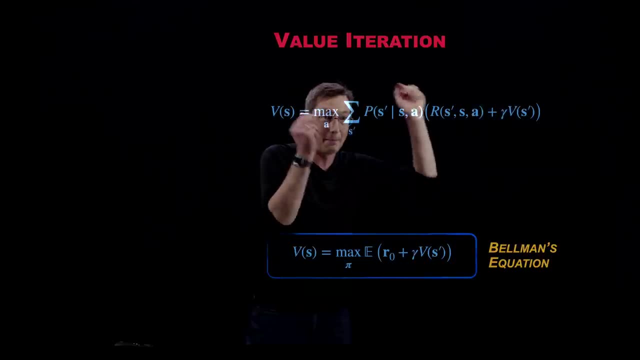 over all actions. I'm going to compute this for all actions and pick the best action that gives me the maximum possible value, assuming this bad estimate here, And I'm going to update the value function at this current state s that I'm currently at. 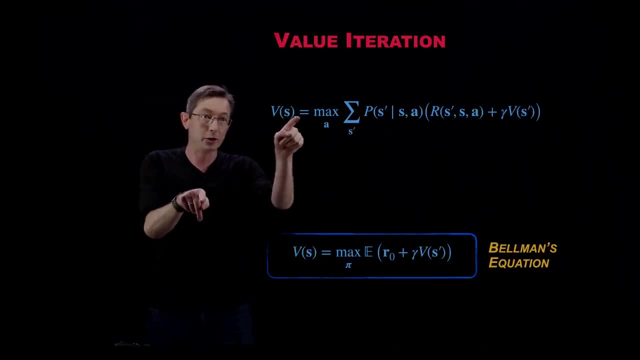 I'm going to take my table, find my current state and I'm going to update that value function with this maximum expected future reward. Then I take the next step and I do the whole process again, And I take the next step and I do the whole process again. 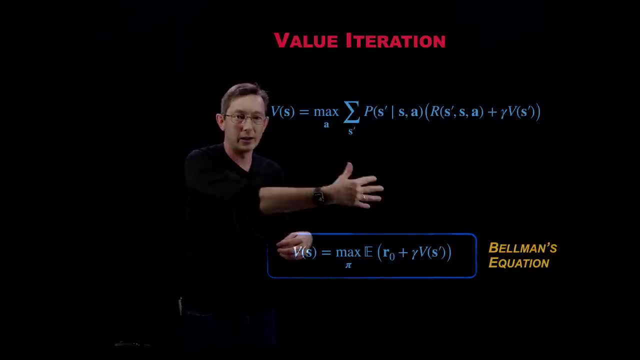 I start there and I start kind of playing the game. I start running through action sequences and updating my estimate of the value function. So let's see how this works. I'm in a state S now and what I'm going to do. 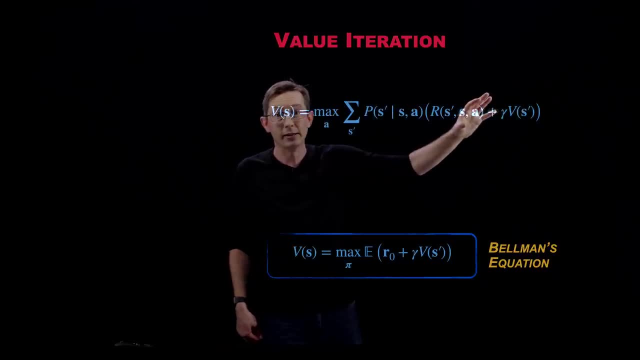 I actually can evaluate this function for all actions Because I know the reward function, I know the model P and I at least have a table of what I think the optimal value function is at all next states. Now that might be a really crummy estimate. 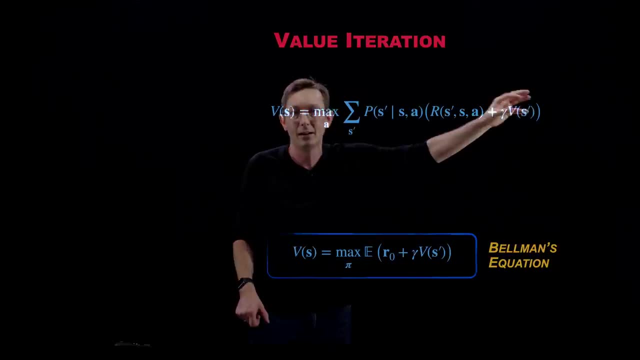 This is kind of a V hat. This is an estimate of the value function. It might be a garbage estimate, but it's something that's the best I've got, And so what I'm going to do is I'm going to maximize over all actions. I'm going to compute this for all actions. 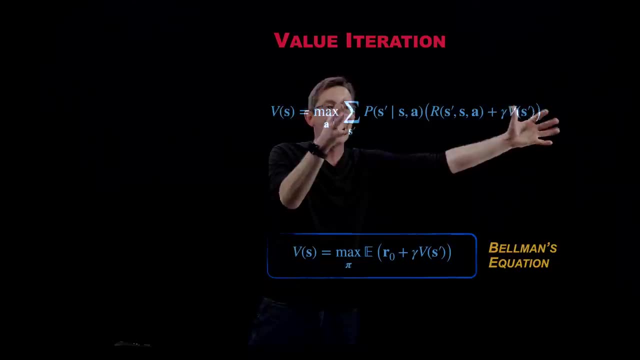 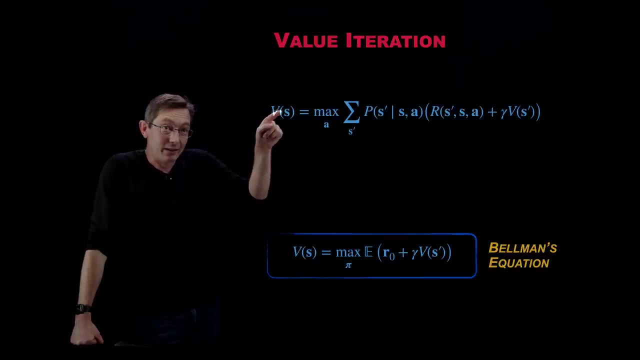 and pick the best action that gives me the best action. So I'm going to do that. This gives me the maximum possible value, assuming this bad estimate here, And I'm going to update the value function at this current state S that I'm currently at. 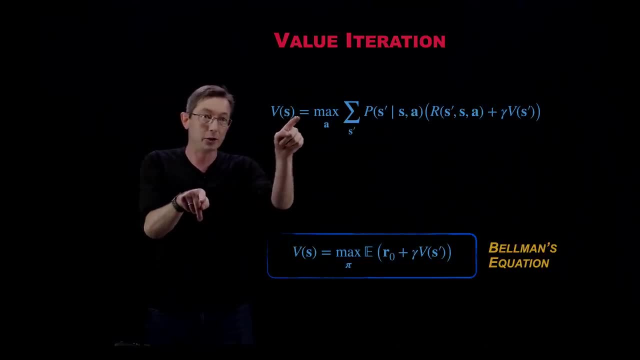 I'm going to take my table, find my current state and I'm going to update that value function with this maximum expected future reward. Then I take the next step and I do the whole process again. Now I'm in a new state and I find the best action. 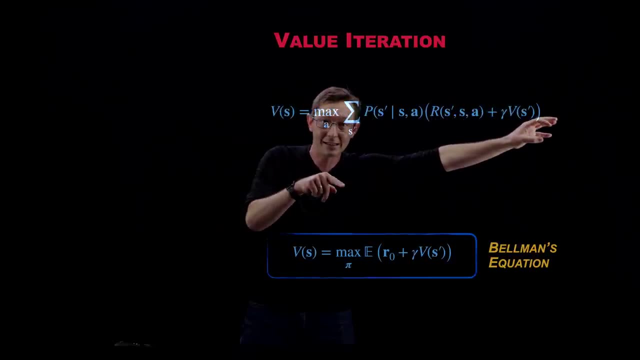 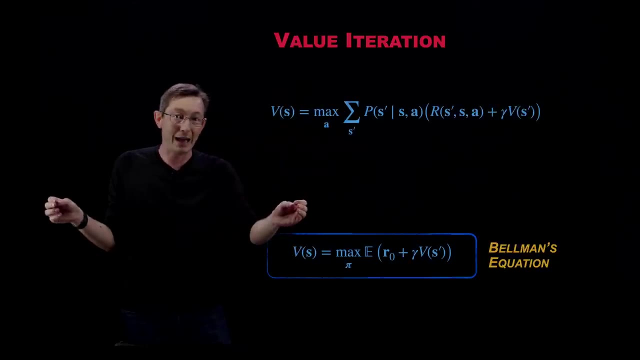 You know, this assumes that I have some estimate of what my value function is at the next state. and I do this again and again, and again, And even if this value function was initialized badly, when I run through this time and time and time again, 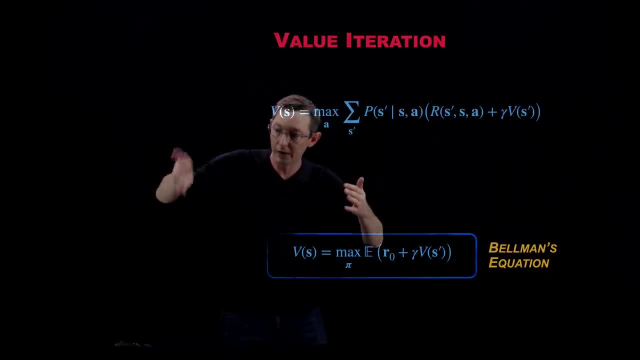 I'm going to iterate through this. That's why it's called policy iteration. I iterate through the game. I play a game of chess, I play another game of chess, and another one, and another one, and another one, And each time I'm updating my value function. 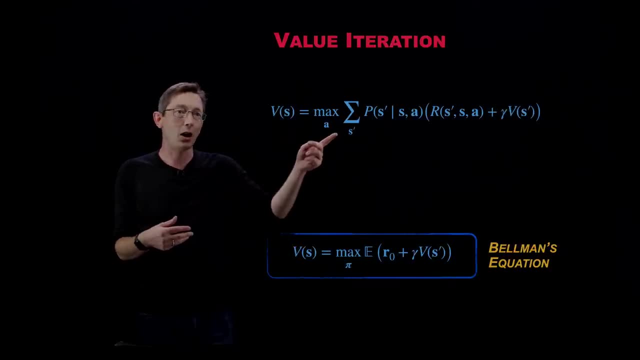 based on what I think is the best action. This is on policy. This is on policy, if you like. And so, eventually, that value function starts to get better and better and better, And the better the value function gets, the better I'm able to update my value function. 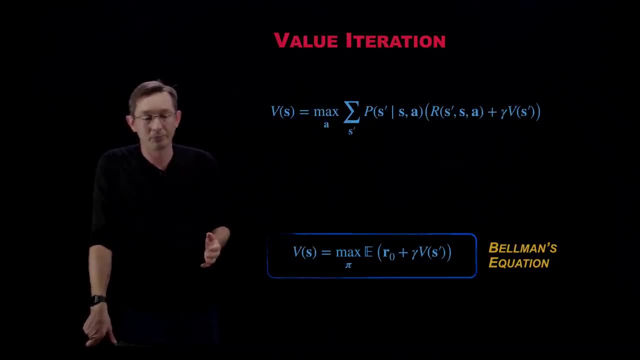 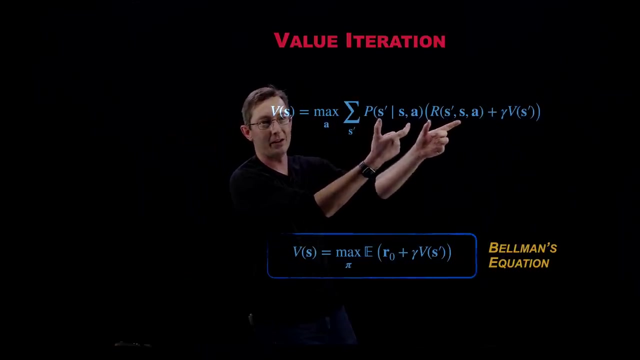 because this is a recursive formula. It's a really simple idea. Because it's recursive, I can just initialize everything poorly and then iteratively kind of refine that value function as I play the game and play the game, and play the game And I'm kind of virtually playing the game, you know. 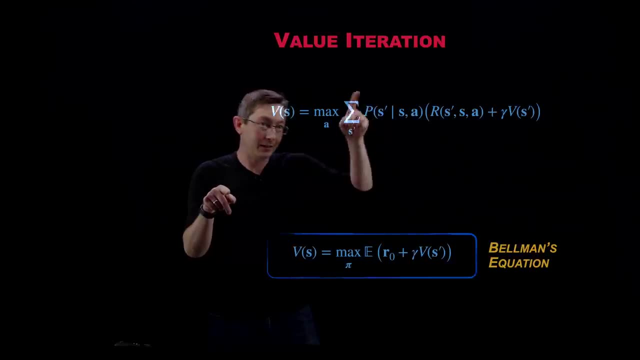 And I take the next step and I do the whole process again, And now I'm in a new state And I find the best action. you know, this assumes that I have some estimate of what my value function is at the next state. 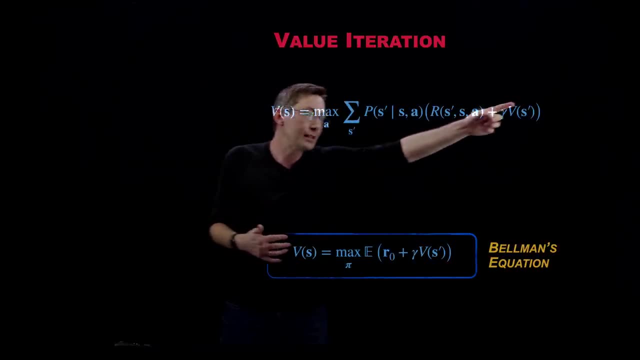 And I do this again and again and again, And even if this value function was initialized badly, when I run through this time and time and time again, I'm going to iterate through this. That's why it's called policy iteration. I iterate through the game. 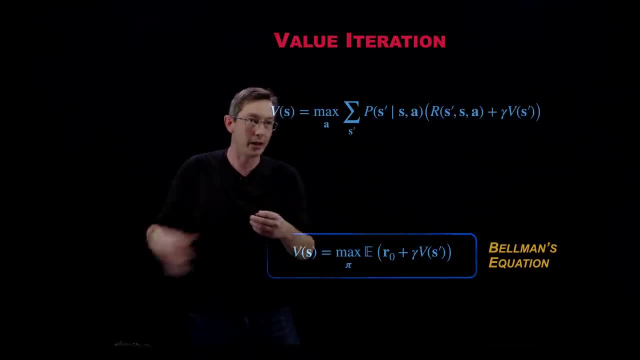 I play a game of chess, I play another game of chess, and another one, and another one, and another one. Each time, I'm updating my value function based on what I think is the best action. This is on policy, if you like. 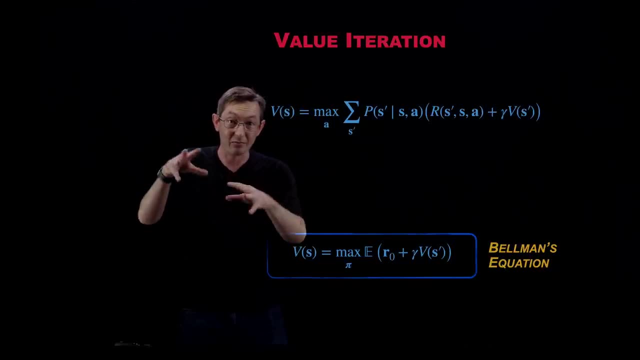 And so eventually, that value function starts to get better and better and better. And the better the value function gets, the better I'm able to update my value function, because you know this is a recursive formula. It's a really simple idea. 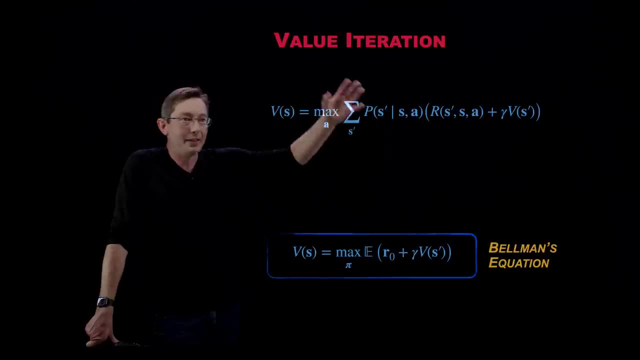 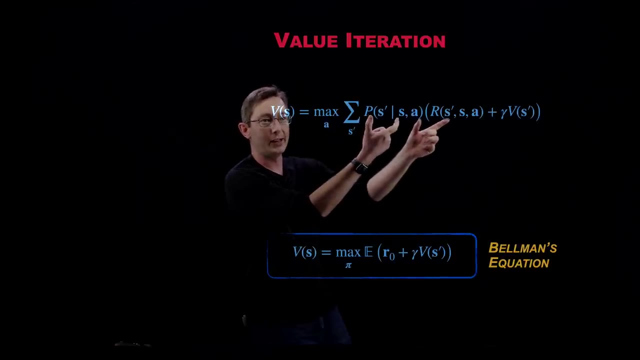 Because it's recursive. I can just initialize everything poorly and then iteratively kind of refine that value function as I play the game, and play the game, and play the game And I'm kind of virtually playing the game. you know a simulated version. 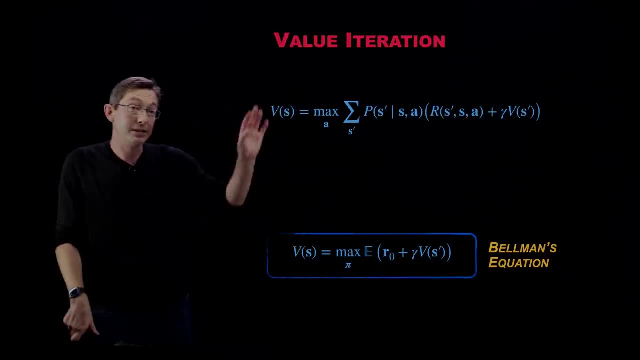 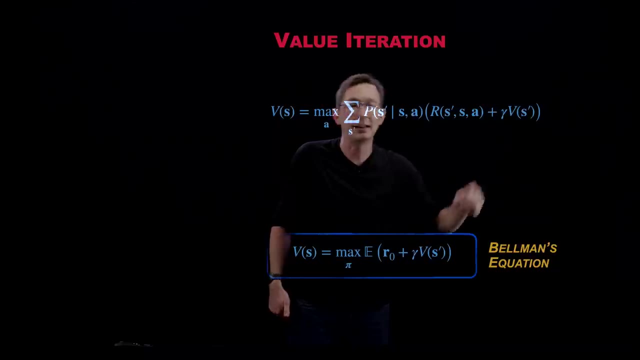 because I know the rules and I know the probability here. So this has to be. you have to have a model to do this value iteration. You need to know p and you need to know what is the expected s prime, the next state, given that p. 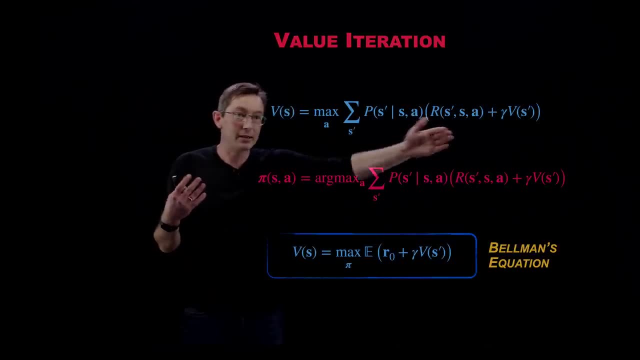 Now, in this case, once I've done this- so I iterate over my policy- I play a game and then I reiterate: I play another game and I play another game- Maybe I start from different random board positions- and then I play, and I play, and I play. 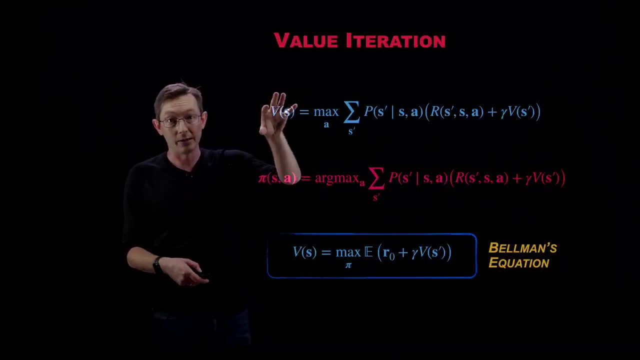 And I iterate until this converges to within some tolerance. Now again, you can't do this for exceedingly large problems, where the state space is, you know, billion or trillion, or 10 to the 80, like in chess, But for small problems like tic-tac-toe. 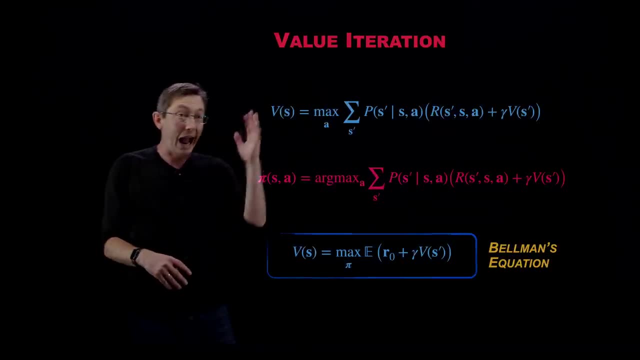 you can actually code this up and try it yourself, Okay, so I highly encourage you to enumerate all of the states of a tic-tac-toe, all of the states of a tic-tac-toe board, and just initialize some crappy random initial value. 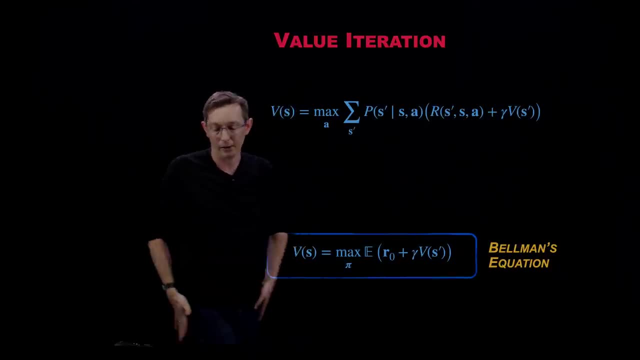 a simulated version because I know the rules and I know the probability here, So this has to be. you have to have a model to do this value iteration. You need to know P and you need to know what is the expected S prime. the next state, given that P. 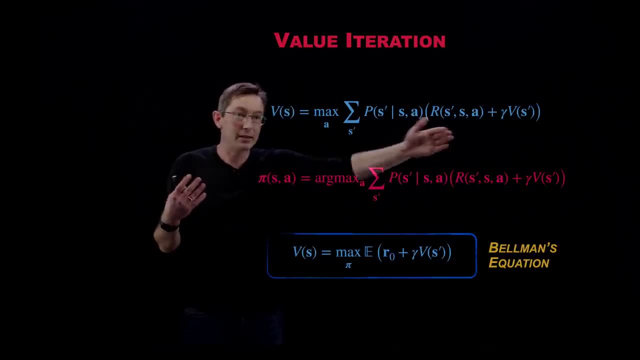 Now, in this case, once I've done this- so I iterate over my policy- I play a game and then I reiterate: I play another game and I play another game. Maybe I start from different random board positions and then I play. 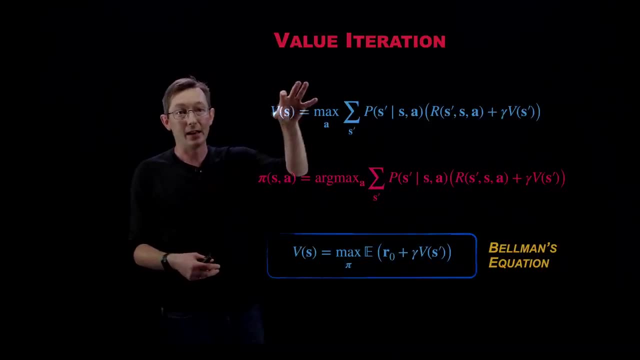 I play, and I play, and I play And I iterate until this converges to within some tolerance. Now again, you can't do this for exceedingly large problems where the state space is, you know, billion or trillion, or 10 to the 80, like in chess. 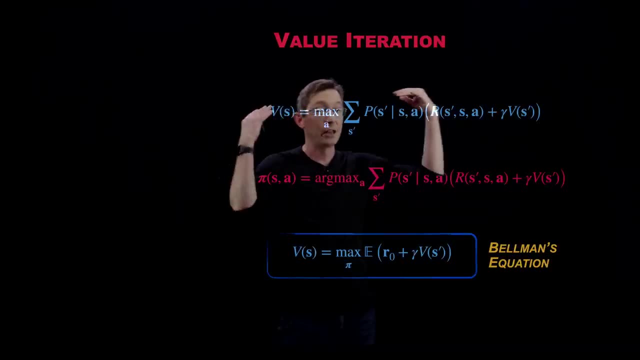 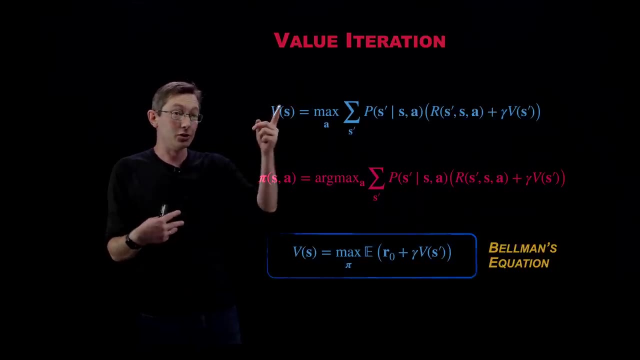 But for small problems like tic-tac-toe, you can actually code this up and try it yourself, okay. So I highly encourage you to enumerate all of the states of a tic-tac-toe board and just initialize some crappy random initial value to every possible state. 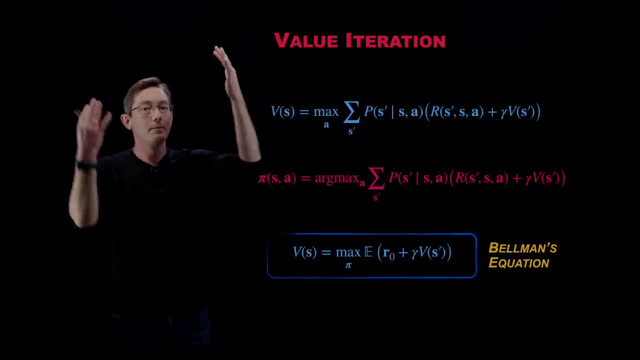 And then run through this value iteration, some big for loop, until you refine that estimate And once that's converged you can then extract the optimal policy as the A that maximizes this thing. you've been working with this thing here, So that's value iteration. 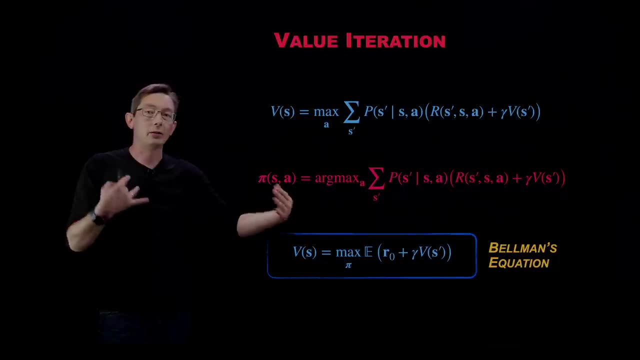 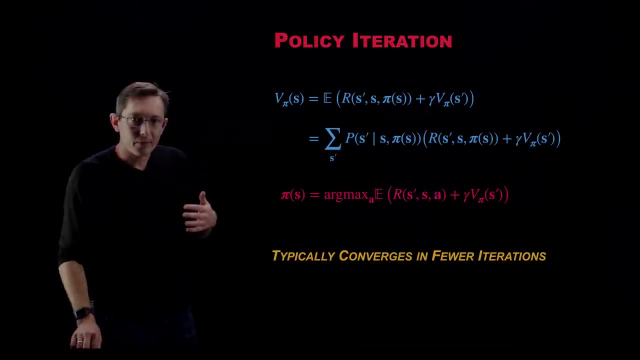 And this relies on Bellman's optimality condition and it uses dynamic programming. It's a type of dynamic programming, So the kind of other leading approach that was value iteration Policy. iteration is just a little bit more complicated but also very similar. 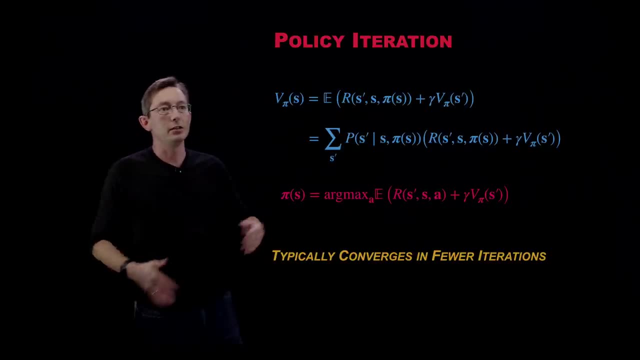 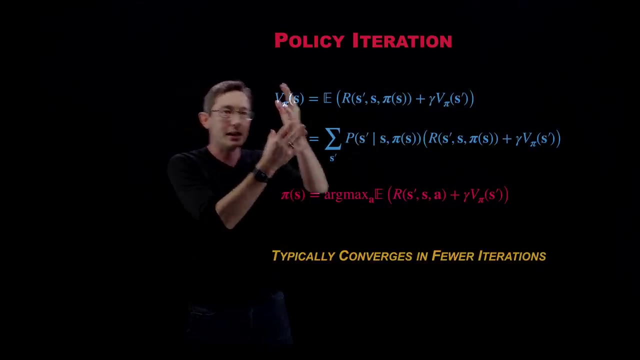 And it's a two-step iteration process. So what we do is: the first thing is we lock in a policy pi, So it's whatever we think is the best policy pi, And we iteratively update our value function locking in that policy pi. 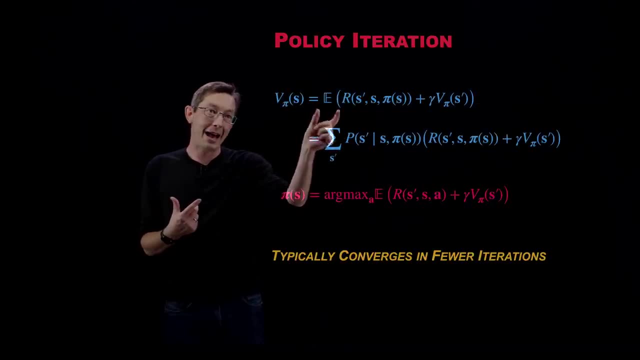 So we do the exact same thing as before, but instead of doing the max overall actions A, we just enact our whatever we think our best policy is And again we kind of iteratively update what the value is for every state by walking through different states. 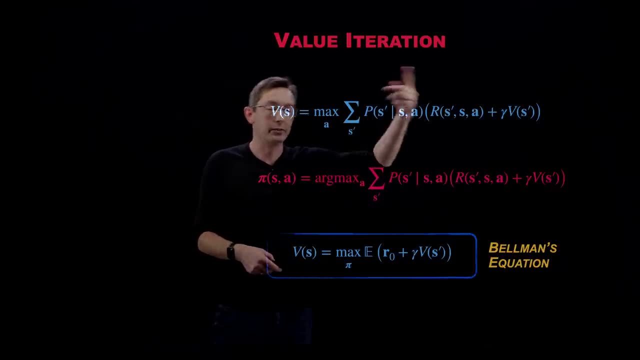 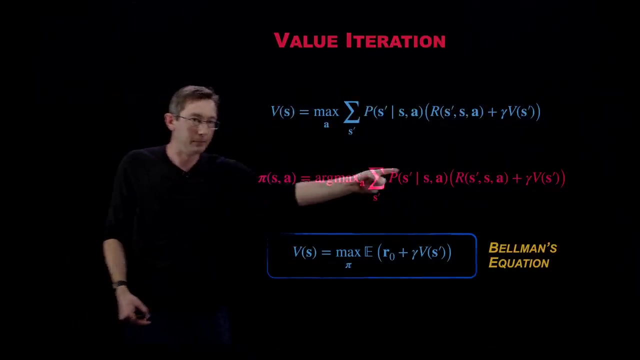 to every possible state and then run through this value iteration, some big for loop, until you refine that estimate And once that's converged you can then extract the optimal policy as the a that maximizes this thing you've been working with. 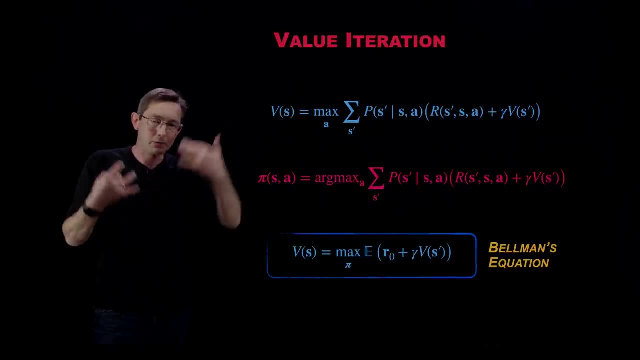 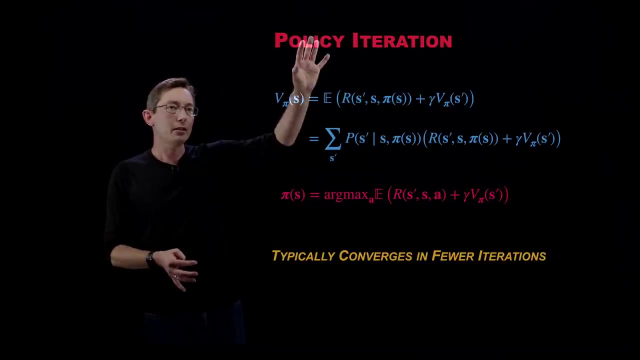 this thing here. So that's value iteration And this relies on Bellman's optimality condition and it uses dynamic programming. It's a type of dynamic programming, So the kind of other leading approach that was value iteration Policy iteration is just a little bit more complicated. 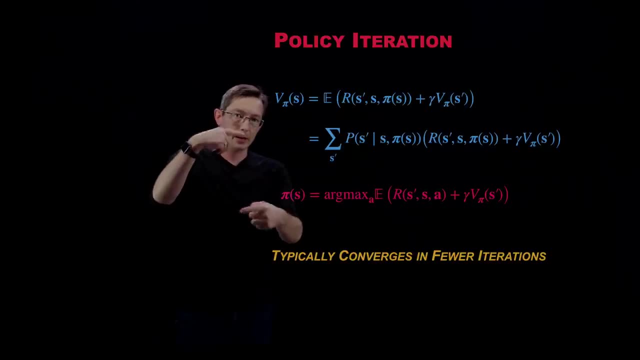 but also very similar, And it's a two-step iteration process. So what we do is: the first thing is we lock in a policy pi, So it's whatever we think is the best policy pi, And we iteratively update our value function. 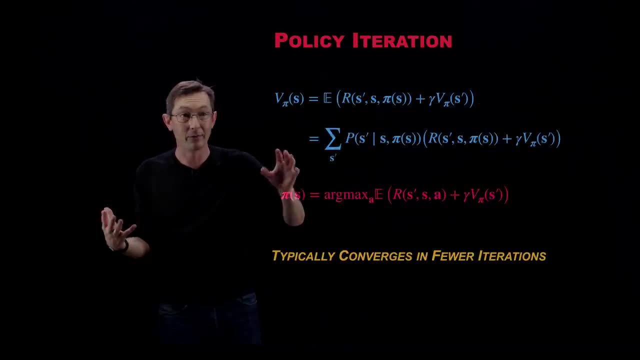 locking in that policy pi. So we do the exact same thing as before, but instead of doing the max overall actions a, we just enact our whatever we think our best policy is And again we, you know, kind of iteratively update what the value is for every state. 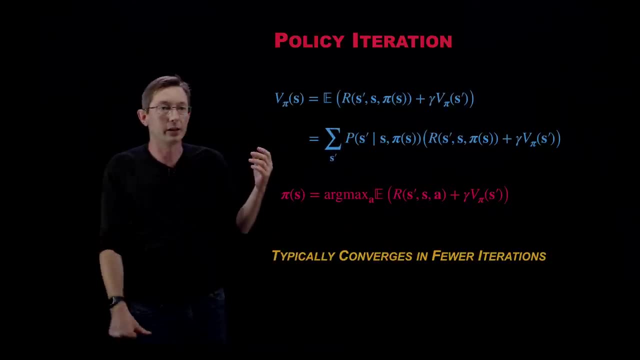 by walking through different states and seeing what happens essentially, And then we lock in that value function. after we've iterated on that, we lock in the value function and then we sweep through the action. we lock in the value function And then we sweep through the action. 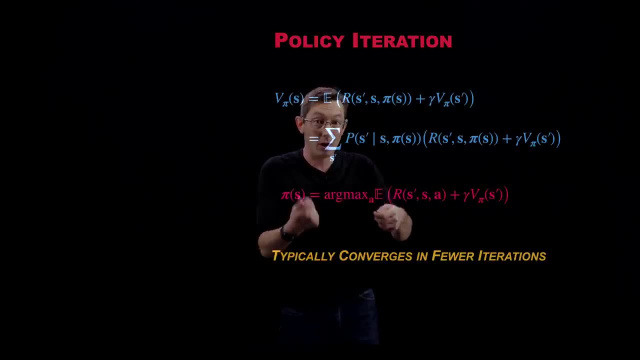 and then we sweep through the action, actions and we try to iteratively update the policy so that, given a state S, we can take the best actions A that maximize our future rewards. Now again, that assumes that I have a good working model of my value function at this state and at all future states, at the next state S prime. 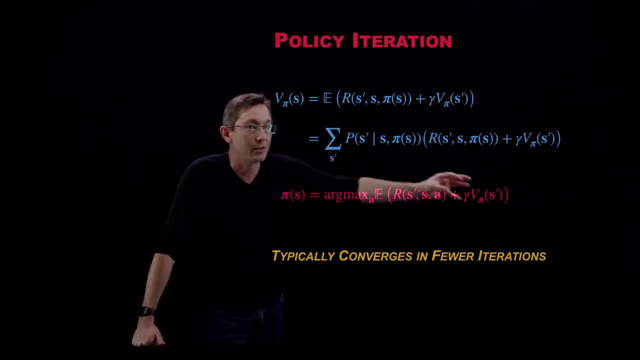 Now again, this might be a bad approximation of the value function here, but it's usually good enough to improve my policy. Then, once I improve my policy, I lock my policy and I do another value iteration step And that might be still a crappy policy and a bad estimate. 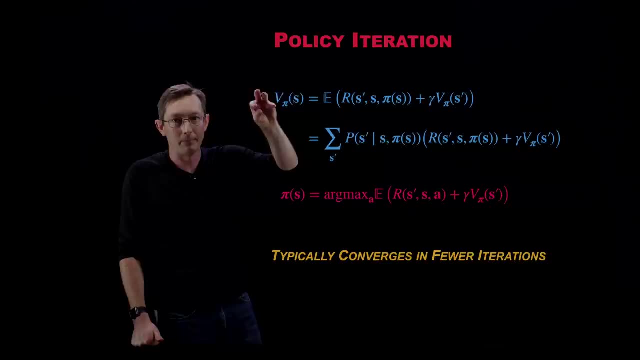 of the value. but it's good enough to improve my value function. And now, based on that better value function, I lock that in and I improve my policy. Based on that policy, I improve my value function. And this iterative procedure: again, you iterate until some convergence criteria. 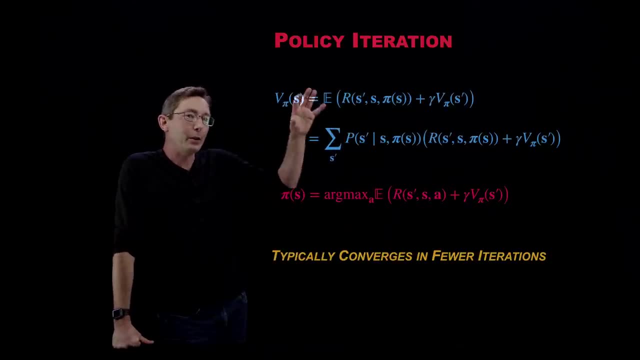 and seeing what happens essentially And then we lock in that value function. after we've iterated on that, we lock in the value function And then we sweep through the actions and we try to iteratively update the policy so that given a state S. 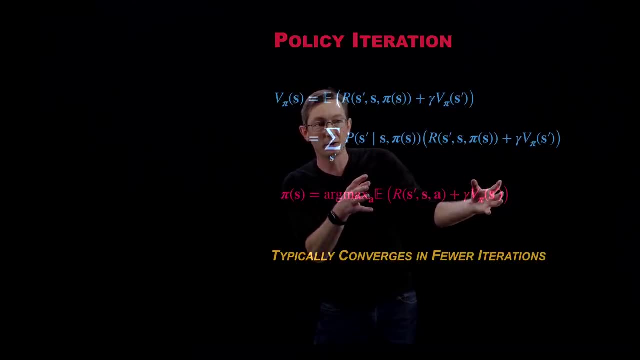 we can take the best actions A that maximize our future rewards. Now again, that assumes that I have a good working model of my value function at this state and at all future states at the next state S prime. Now again, this might be a bad approximation. 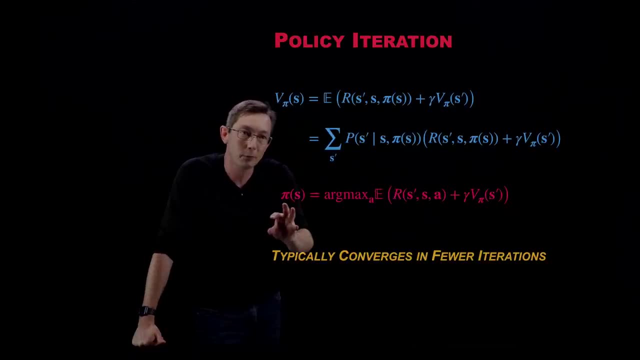 of the value function here, but it's usually good enough to improve my policy. Then, once I improve my policy, I lock my policy and I do another value iteration step And that might be still a crappy policy and a bad estimate of the value. 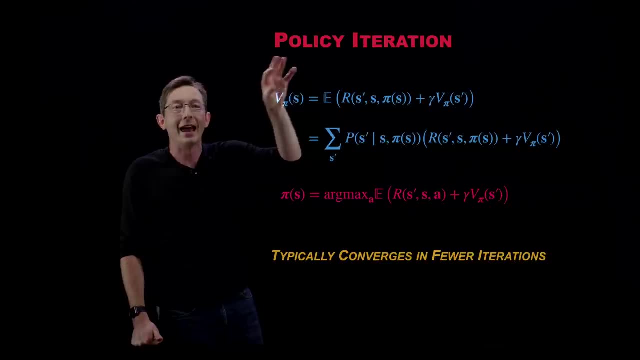 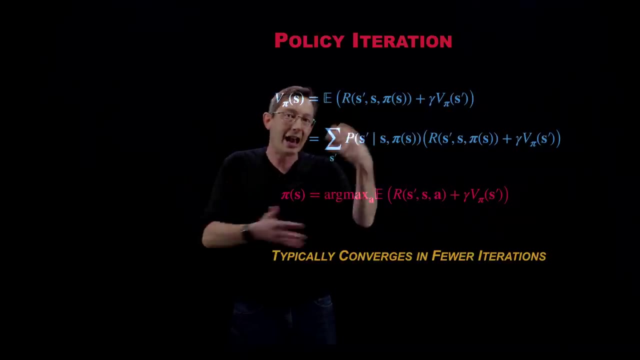 value. but it's good enough to improve my value function. And now, based on that better value function, I lock that in and I improve my policy. Based on that policy, I improve my value function. And this iterative procedure: again, you iterate until some convergence. 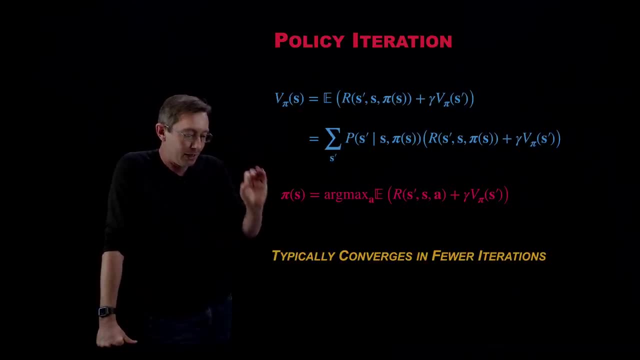 criteria. This is a lot like the kind of alternating directions optimization that we see in machine learning. So policy iteration often converges in fewer iterations than pure value iteration. So this is often kind of a preferred approach in a lot of cases. And again I would like 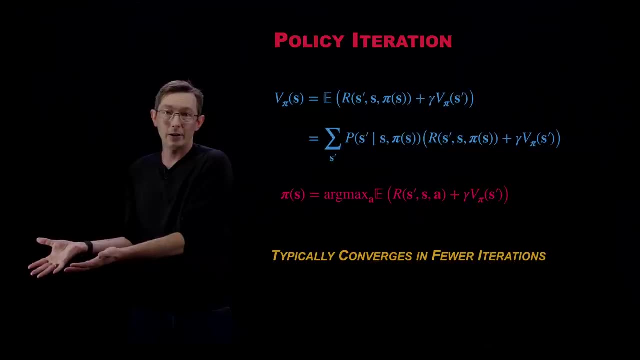 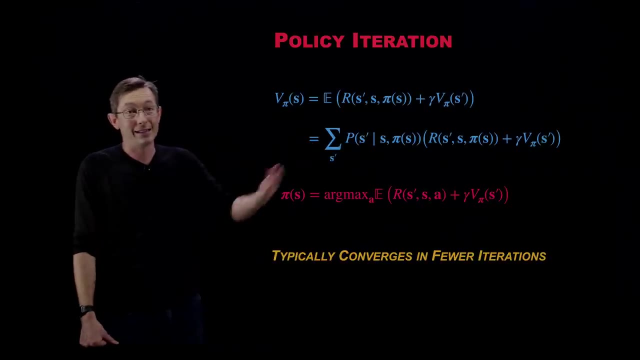 you to try on the game of tic-tac-toe. write a program to do value iteration, write another one to do policy iteration and compare how fast they converge, which one converges in less iterations, which one's faster, you know on your CPU. 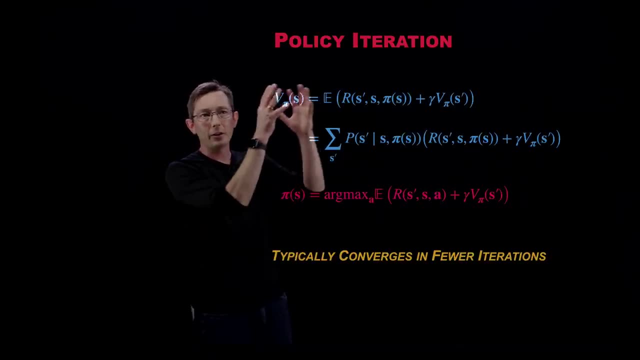 So the last thing I want to talk about is policy iteration. And I want to talk about the last thing I want to point out is that the value function v, where, essentially, you know, optimizing the action to maximize this future expected reward, this expectation here, 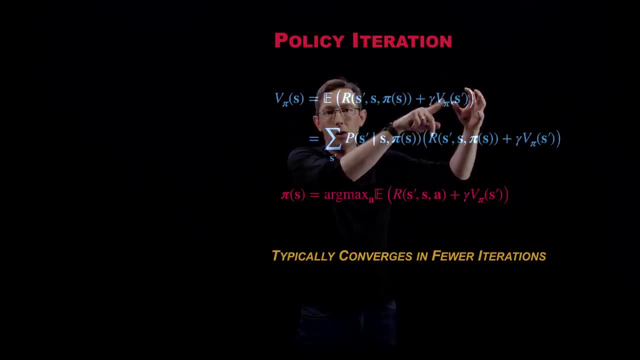 my reward now plus my, you know, discounted all some of my future rewards. And when I compute my policy function pi, I'm also I'm trying to maximize over actions. I'm trying to find the action that maximizes this expectation. 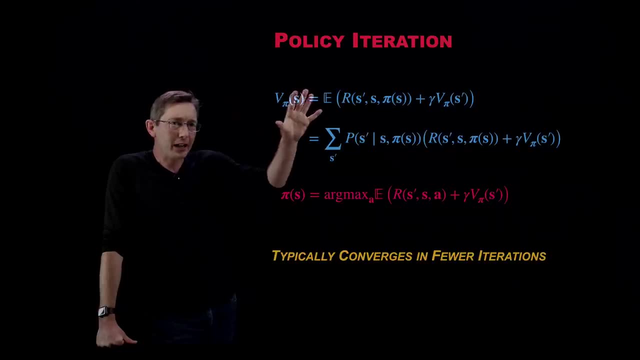 This is a good example of how you can improve your value function. This is a lot like the kind of alternating directions optimization that we see in machine learning. So policy iteration often converges in fewer iterations than pure value iteration. So this is often kind of a preferred approach in a lot of cases And again I would like you to try. 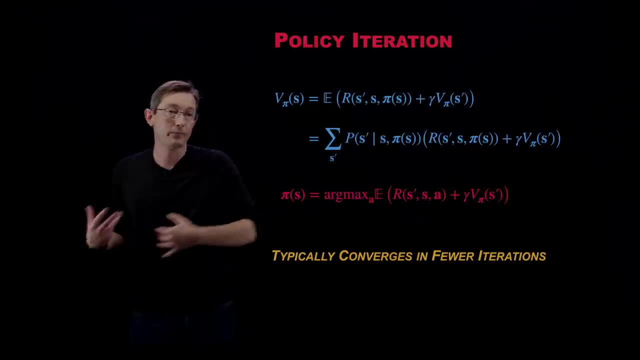 on the game of tic-tac-toe. write a program to do value iteration, write another one to do policy iteration and compare how fast they converge. So this is a lot like the kind of alternating which one converges in less iterations, which one's faster on your CPU. 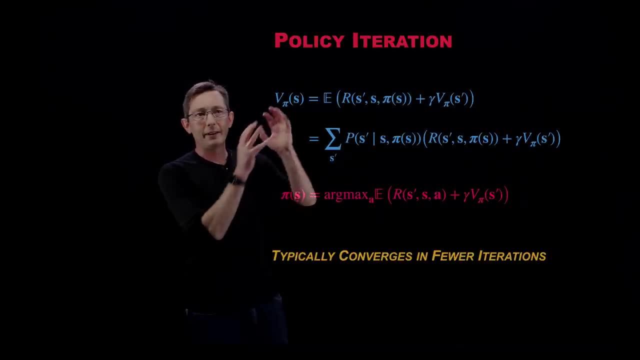 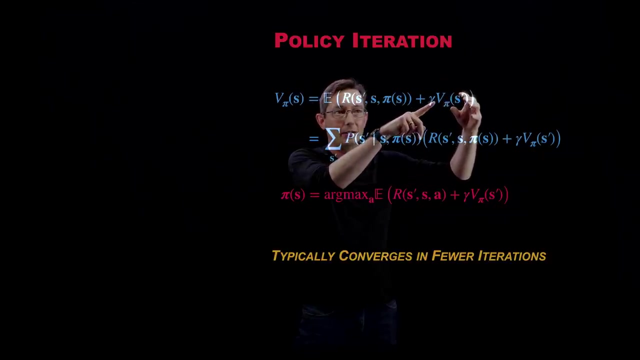 So the last thing I want to point out is that the value function v, we're essentially optimizing the action to maximize this future expected reward, this expectation here, my reward now plus my discounted, all some of my future rewards. And when I compute my policy function, 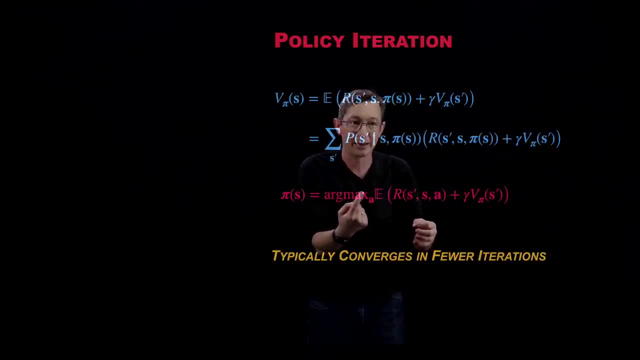 pi. I'm also. I'm trying to maximize over actions. I'm trying to find the action that maximizes this expectation. So it seems like there's redundant information. The value function and the policy function: both are intimately depending on this expectation of all future. 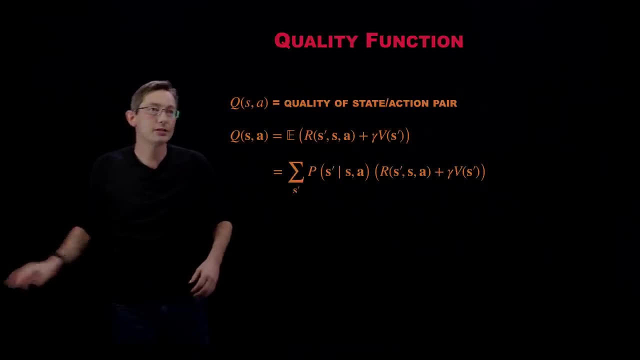 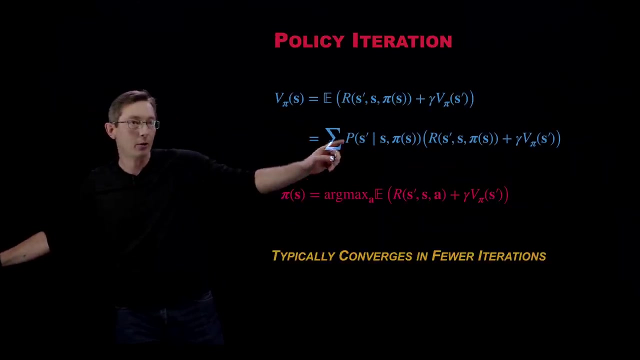 rewards here. And so it turns out you can introduce something called the quality function, this Q function, which is the quality of being jointly in a state S and taking an action A, And literally, this quality function is that expectation from before. So this expectation, 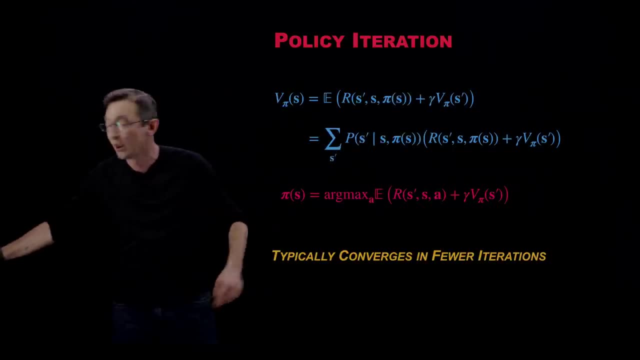 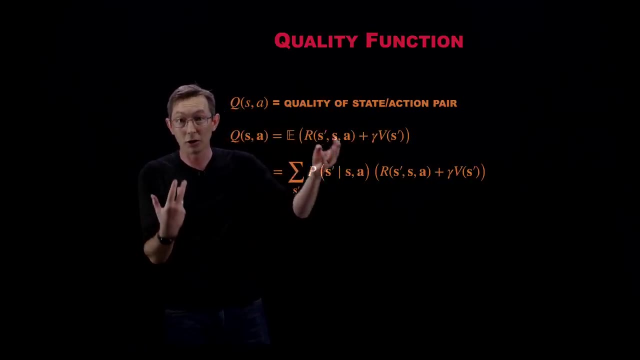 that we're trying to estimate with our value function or exploit with our policy is the quality function. It is the expected future, current and future rewards. given a state S and an action A, Now the Q function. it seems like I've just renamed something I've already. 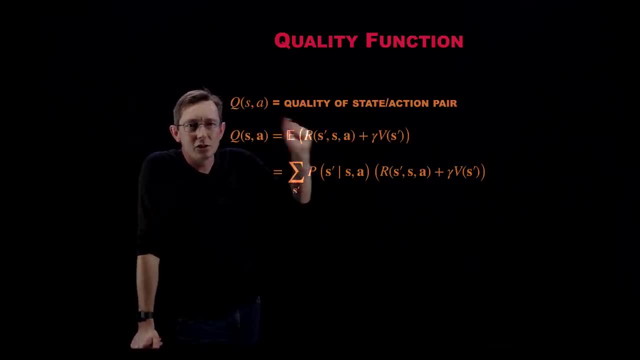 worked with and I have. But this is super, super important because when I did policy iteration and value iteration, I needed to have a model of what my future state S prime is, so that I could use this value at that next state in my optimization, in my recursive dynamic programming optimization. 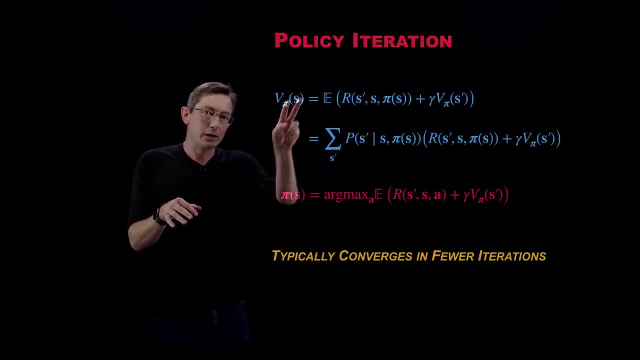 So it seems like I'm going to be able to do this, And I'm going to be able to do this with the value function, And I'm going to be able to do this with the value function. So it seems like there's redundant information: the value function and the policy function. 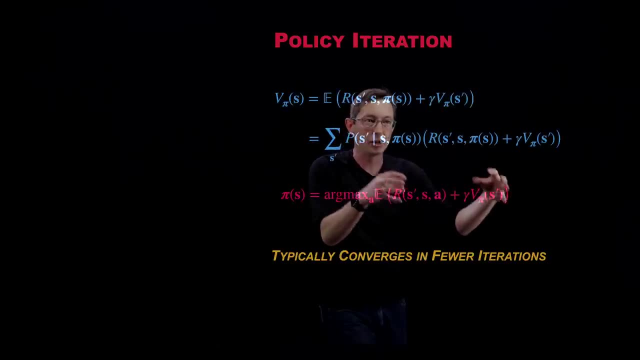 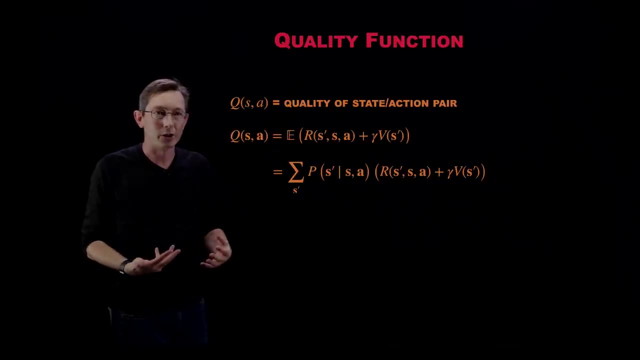 both are intimately depending on this expectation of all future rewards. here, And so it turns out, you can introduce something called the quality function, this Q function, which is the quality of being jointly in a state S and taking an action A, And literally this: 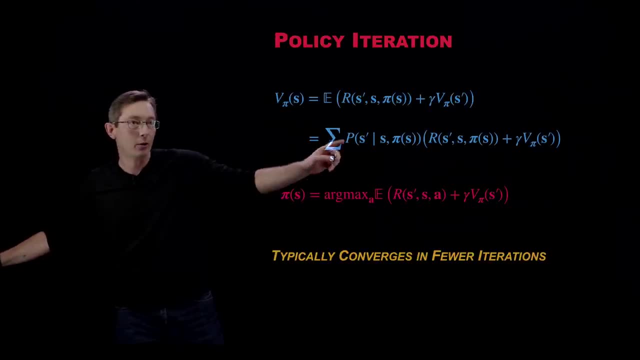 quality function. is that expectation from before. So this expectation that we're trying to estimate with our value function, we're going to be able to do this with the value function And so it seems like I'm going to be able to do this with the value function And literally this: 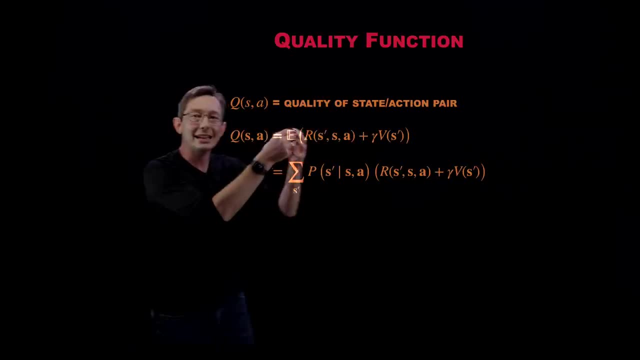 is the quality function, It is the expected future, current and future rewards given a state S and an action A. Now the Q function. it seems like I've just renamed something I've already worked with and I have, But this is super, super important, Because when 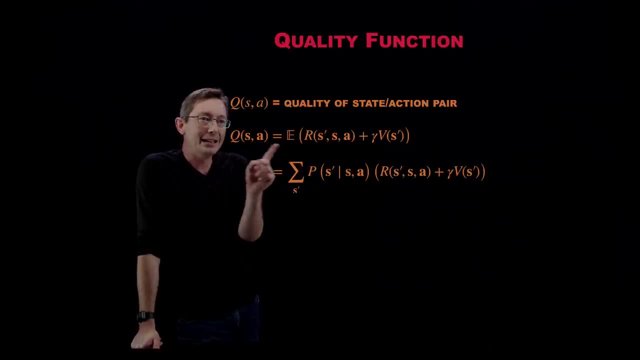 I did policy iteration and value iteration. I needed to have a model of what my future state would look like, And so I'm going to be able to do this. with the value function, The option is to make the state S prime is, so that I could use this value at that. 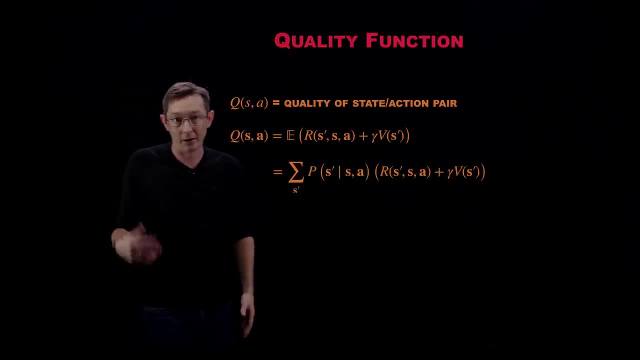 next state in my optimization, in my recursive dynamic programming optimization, Whereas in the quality function, if I start to learn a quality function, Q of S and A, all of this information is implicitly in this function And so I can optimize directly and learn. and 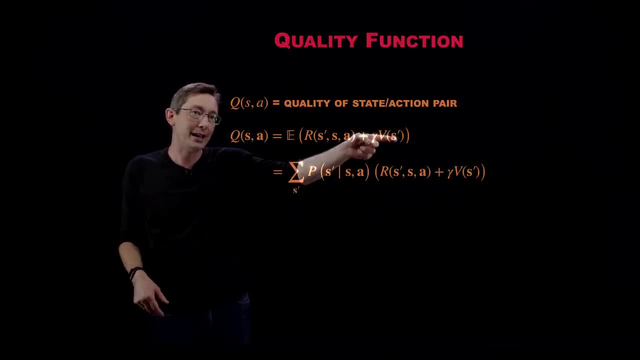 iteratively improve it, And I don't need a model for what my next state is, because it's already implicitly defined, And so I can do that, And so I can do that, And so I can find in the quality function. That's a subtle point, but this quality function, just writing. 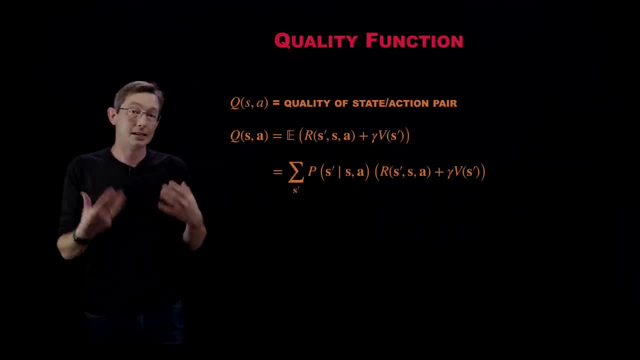 it, so it's implicitly a function of the future state. instead of an explicit function means that I can do model-free reinforcement learning. I can optimize this quantity directly without knowing what my future state is going to be. I can do this by trial and error And again from this quality. 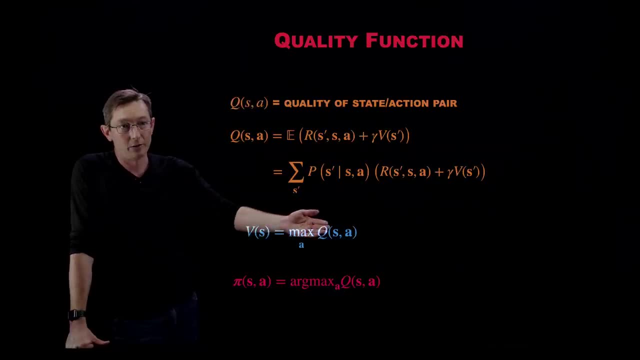 function. once I learn a good quality function, I can extract my value function or my policy pi from this Q function. So this has all the information I need to get my value function or my optimal policy. And so it's evolving that lots and lots of modern reinforcement learning.